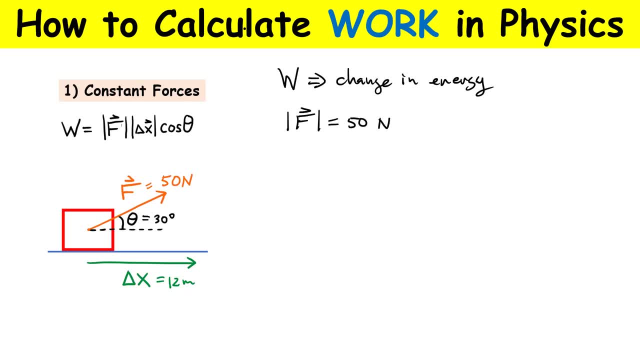 Okay, the next thing is: what is the magnitude of my displacement vector? Well, my vector goes in this direction, goes to the right. So the magnitude of that displacement in this case is 12 meters. okay, And the last term is simply cos of the angle, theta. 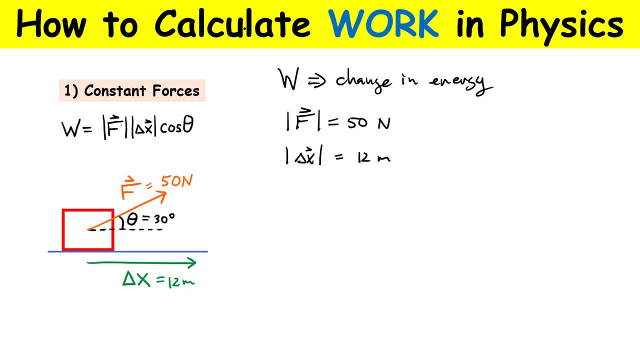 Now, in order for you to really get this right. okay, this is an important point For this operation here, this angle theta, what you're going to want to do is you're going to want to get this right, So you're going to want to get this right. 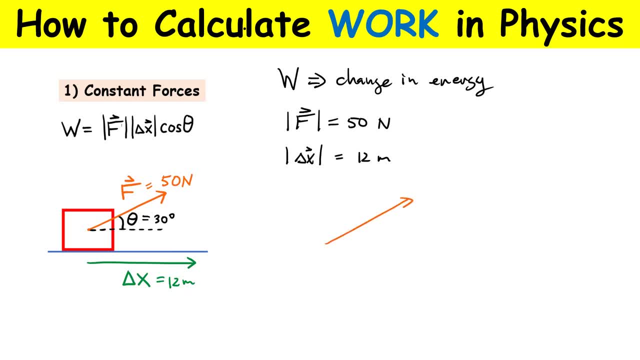 This angle, theta. what you have to do is you have to put the vectors starting at the same position, okay, so that's kind of an important point. So I put my force here. I have my displacement, delta x, which is 12 meters here. 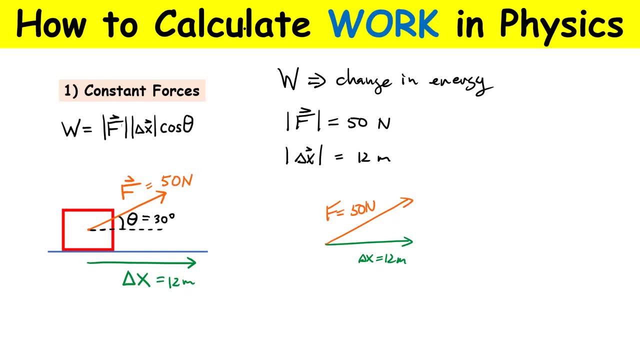 You see, if I place those vectors starting at the same point, the angle theta is always the angle between both of the vectors. So in this case it's pretty straightforward: It has to be 30 degrees. So if I wanted to calculate the work done by this 50 Newton force, 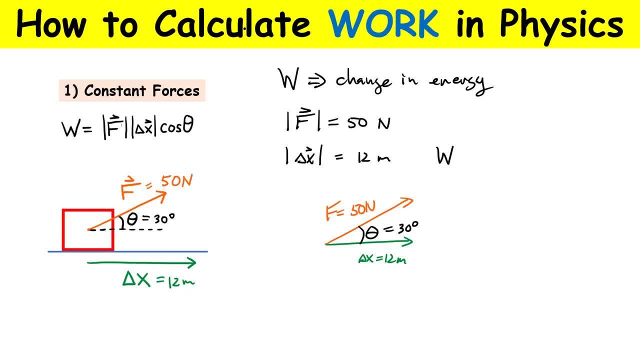 All you do now is apply this formula. All right, so you'd say the work is equal to the magnitude of the force: 50, positive number. The magnitude of the displacement is going to be 12,. okay, And cos of the angle between both the force and the displacement. 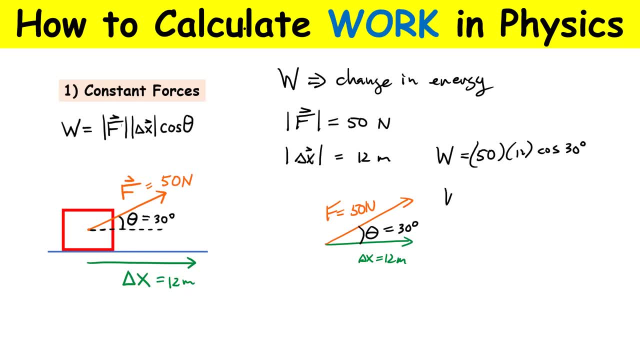 So you have cos of 30 degrees. All right, you put that in the calculator and you should get a number of 519.6.. Now the units end up being Newtons for the force And meters for the displacement. Cos of the angle doesn't have units. 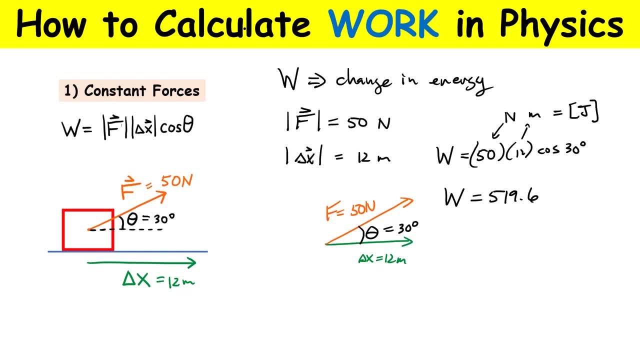 And this is what you call a joule. okay, And Newton times a meter ends up being a joule. All right, if you wanted to just round that to say two significant figures, I would say it's 520 joules Would be the amount of work done by that force F. 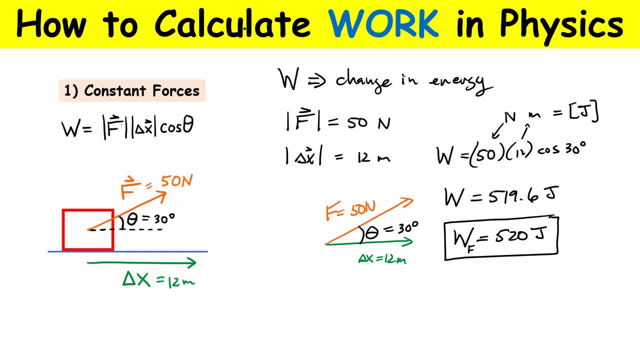 Sometimes I'll add a little subscript there just to remind me that I'm doing it by this force. All right now, this is only valid for constant forces. Now there are other forces acting on this block here as it's sliding across the table. 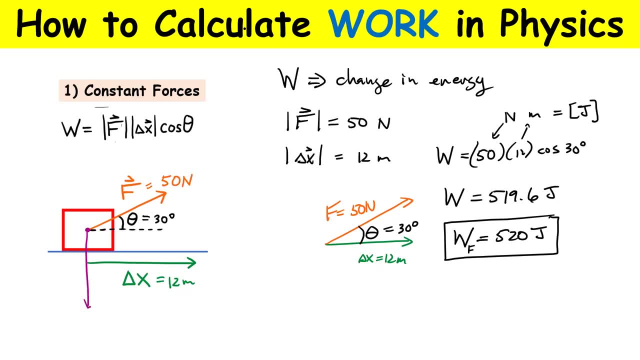 For example, this block probably has a weight right. The magnitude of the weight is mg, And imagine here the mass was 4.0 kilograms. Now what else could we have? Well, we could also have a normal force right. 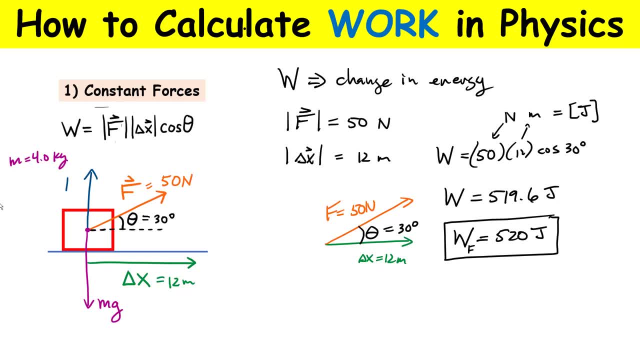 There would be a normal force of the ground pushing up- I'm just going to call that n- And we could calculate what that value is. But that's another example of a constant force. Now, if that object was sliding on the table, guess what? 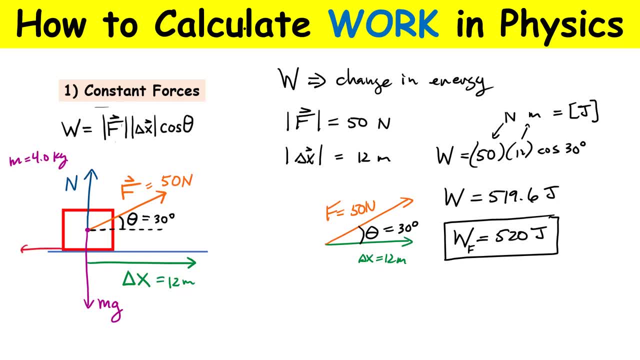 There could also be a force of friction. All right, there might be a force of kinetic friction between the block and the ground. Okay, that might also be a constant force. So let's now add a few forces and see how we would calculate the work done by any of these constant forces. 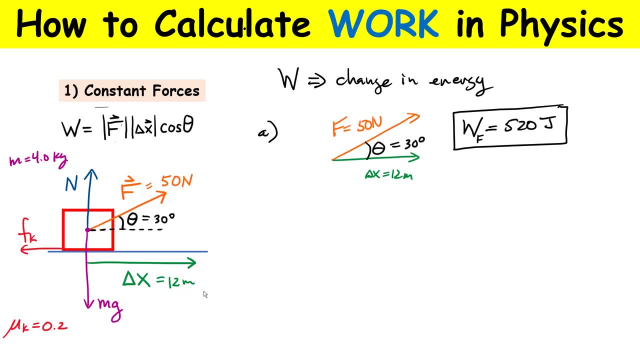 So we've got the work done by the force F, which 50 Newton force, That was 520.. All right, let's go ahead now and do the rest of the terms. So the second force we can consider, for example, might be the weight. 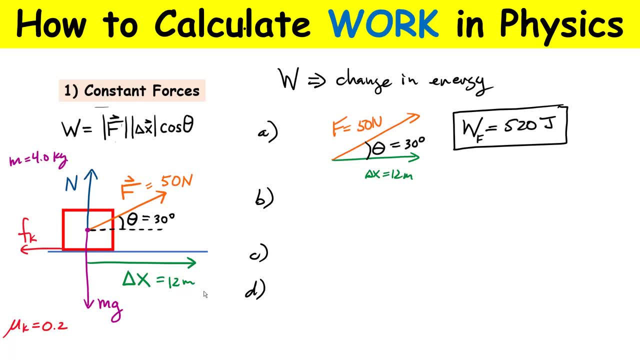 That is a constant force. I could apply this formula: So the work done by the weight. I'll just put a little g here just first to signify the weight. Okay, it's equal to well. what's the magnitude of the force? 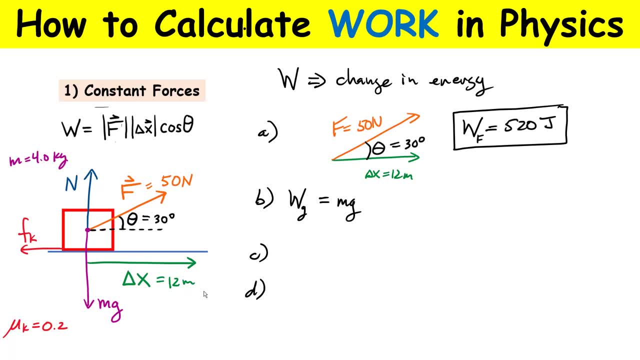 It's mg. It's only positive mg. It's just the magnitude. how big it is All right. what else? Multiplied by the magnitude of the displacement, Again, that's going to be our 12 meters. I'll just write it as delta x. 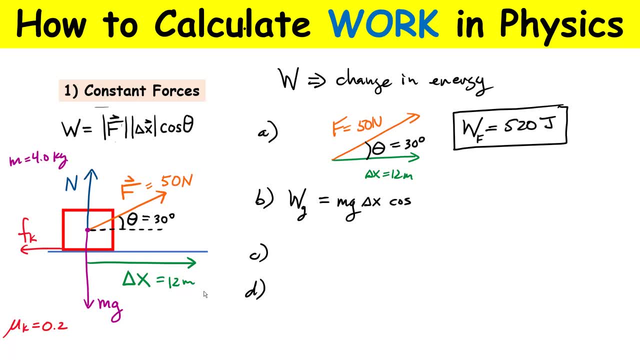 Now multiplied by cos of the angle. Well, what angle would I use here? Okay, what is the angle? Again, the trick is you have to put the vectors end to end. So for this case you have the displacement, which is like this: delta x. 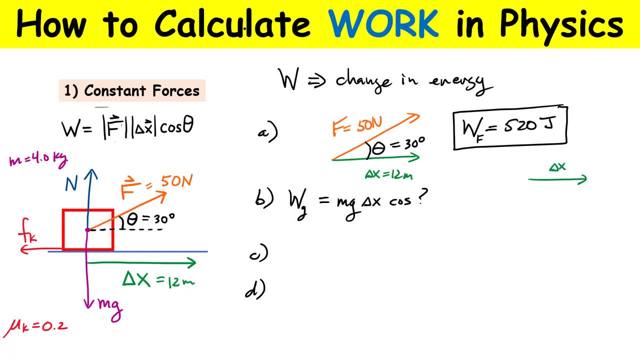 And guess what? I have the weight now which is acting down. Let's switch the color here, but that is the force. All right, what else Now? this is the angle that I'm looking at. So this force in this particular case, what we have is an angle of 90 degrees. 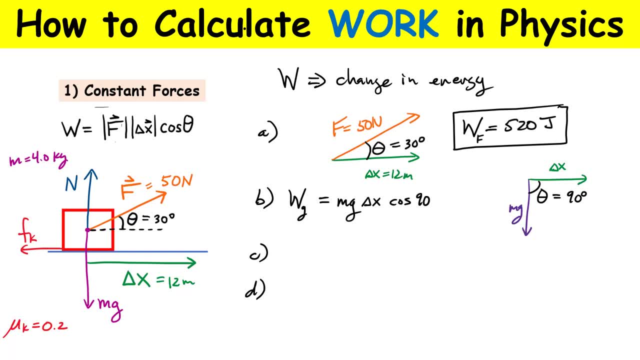 All right, if you don't know that, you can put that in a calculator, but what you're going to find is that this is zero. Okay, so the work done by the weight for this particular problem is zero, and it's because of this final term. 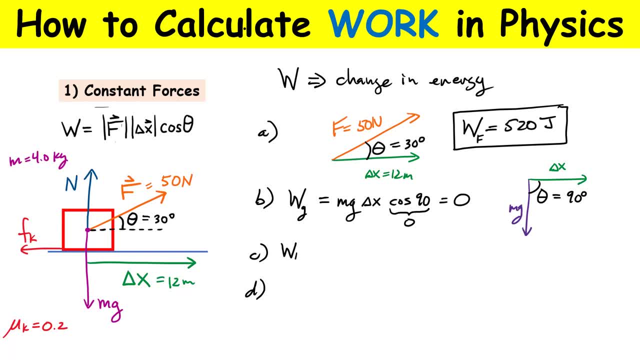 All right, let's look at the other two forces. So we have the work done by the normal force. I'll just call it w, subscript n. It's the magnitude of the normal force, It's the magnitude of the displacement And in this case it's cos of what. 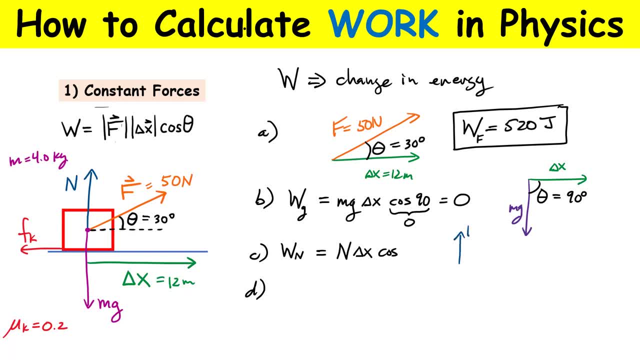 Well, again, putting the vectors end to end. here's my normal force, Here's my displacement. Hopefully this is kind of getting clearer for you now. Again, you see that that angle between this force and that displacement is 90 degrees. 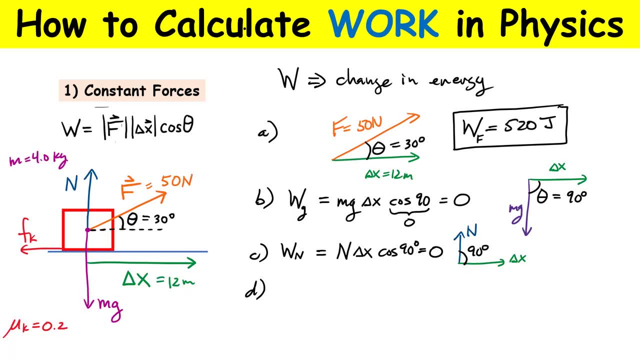 All right. so you do cos of 90, and lo and behold, you get another zero. Well, guess what That means? for this case, the force of gravity doesn't change the energy of the block. It also means that the normal force doesn't change the energy of the block. 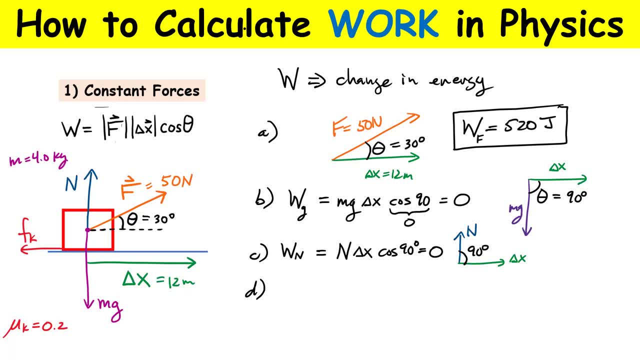 All right, the other force we had here was kinetic friction, because this block here is sliding on the ground and I gave you a coefficient of kinetic friction of 0.2.. Now, if you remember in your physics class, the way you calculate the force is the coefficient of friction. 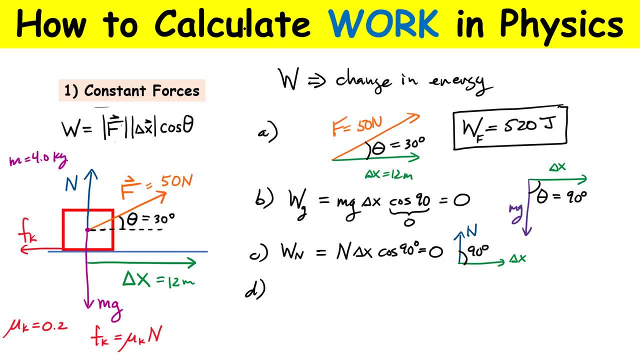 multiplied by a normal force, So we do have to calculate what this normal force is. if I wanted to calculate this force, which I then need to calculate the work done by that force, So how would you calculate the normal force in this case? Now you have to look at all of the components acting in the vertical direction. 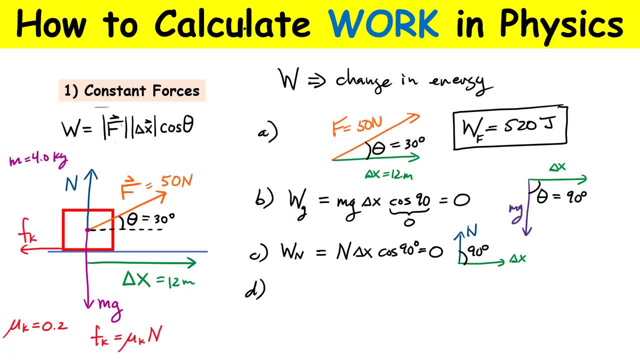 All right, so we're first going to add up all of the components, So you have the normal force and again, that's just applying Newton's first law, right? You add up all the forces in that vertical direction. They have to be equal to 0 because the block is not accelerating up or down. 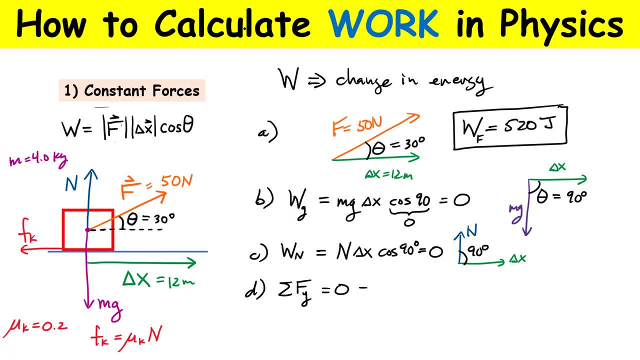 It's only moving in the horizontal distance or direction. So we have the normal force acting up. I'm going to call that plus n, What else? I have the weight acting down, minus mg. All right, now we can't forget about this component, right? 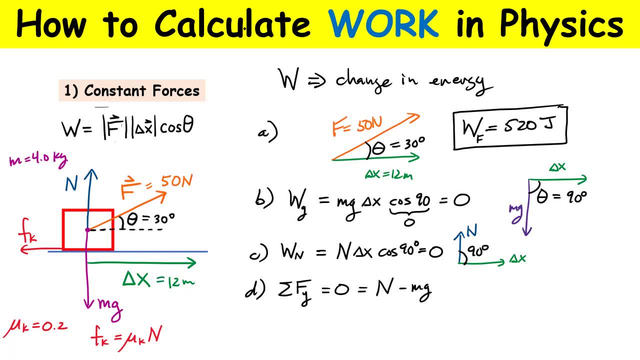 This force, F, does have a vertical component. right, That vertical component is right here and I'm going to call that Fy and that's simply F, F sine of 30 degrees. All right, so if I add that to the Newton's first law, right here again. 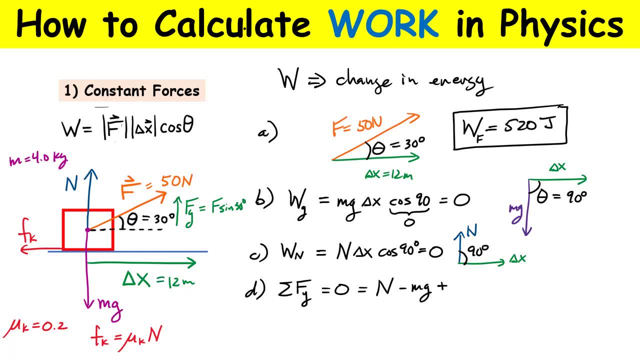 I'm going to assume that that's positive because it's acting up. So here I would have F sine of 30 degrees. All right, that allows me now to solve for the normal force. The normal force, then, is going to be just rearranging this expression minus the weight. 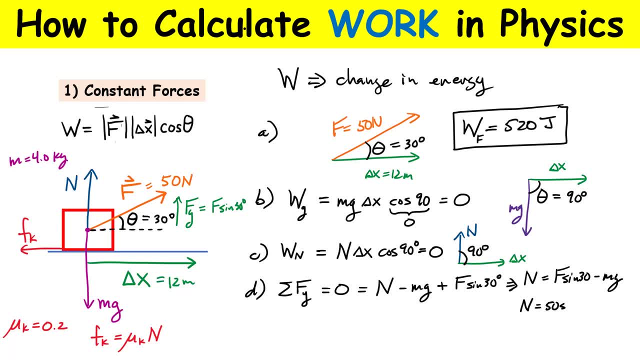 All right, I can put all the numbers in here. So you'll get 50 sine of 30, minus the mass was 4 kilograms And here let's just use 9.8 for little g. So I put that in the calculator and I got a normal force of 14.2 newtons. 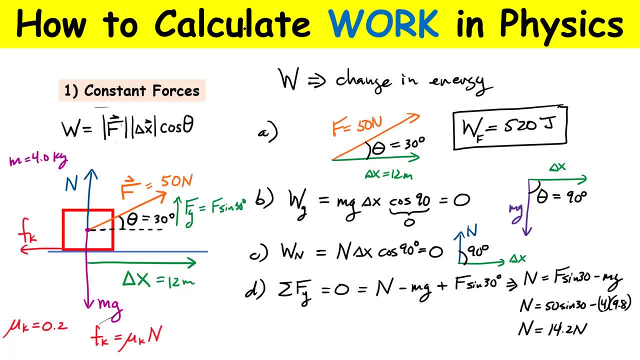 All right, I'm now in a position to calculate what this force of kinetic friction is. right In this case, you just substitute the coefficient 0.2, and multiply it by my normal force 14.2, and I got a force of kinetic friction which is small. 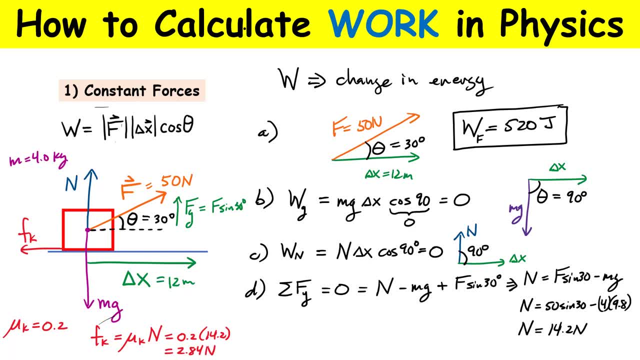 but 2.84 is what I got, newtons. All right, that's the force of kinetic friction. So now I could apply the equation and find the work done by this force, by the kinetic friction force. Guess what It's, the magnitude of the force of friction. 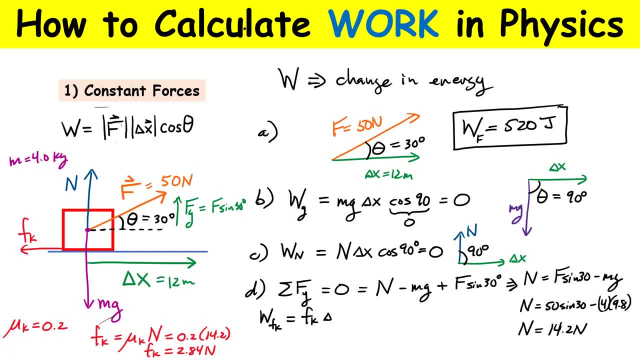 multiplied by the magnitude of the displacement, delta x and the last term, cos of All. right now we have to think about it. What is the angle that I place here for the friction force? Again, the trick that I told you was you have to place the vectors end to end, right. 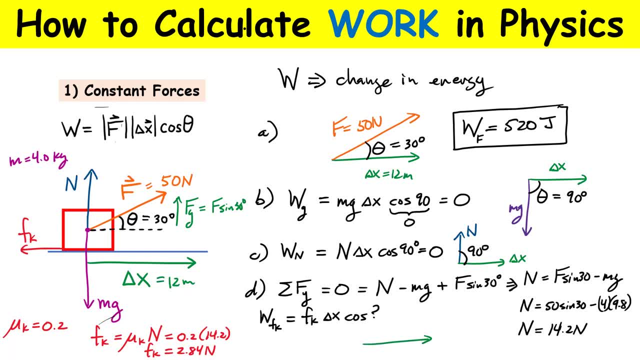 So in this case you have my displacement, which is like this: delta x. I have the force of friction which acts in this direction. here f say sub k, like this, And the angle that goes into my work equation in this case is this angle here. 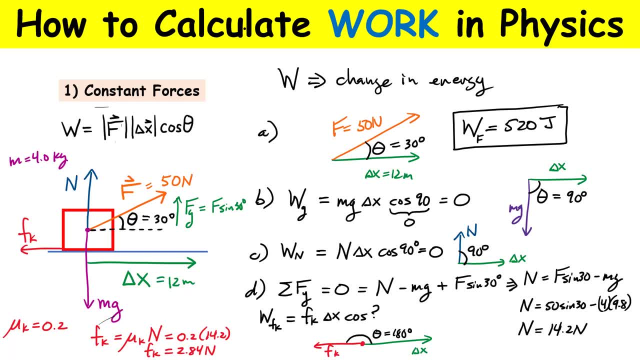 The angle theta is 180 degrees. All right, so you have to substitute 180 degrees right here in the equation for the work. All right, now this one's very important cos of 180.. If you don't remember that one, that one is equal to minus 1.. 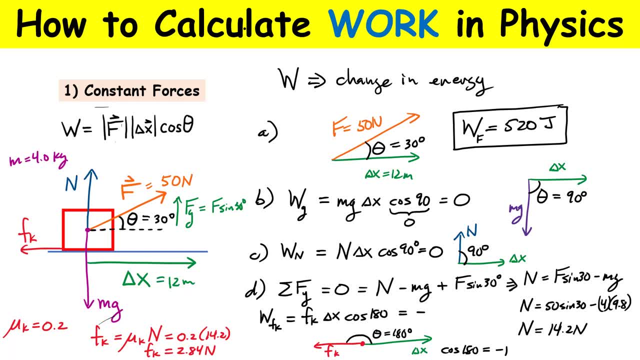 Okay, so all of this then you can simply simplify as minus the force of kinetic friction multiplied by delta x. All right, let me give myself a little bit more space here and we'll finish off this calculation. All we have to do now is just substitute in our numbers. 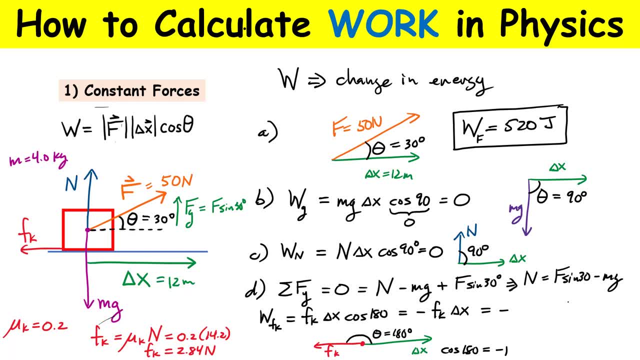 All right. so guess what We get minus. the force of kinetic friction was 2.84 multiplied by 12 meters. Okay, I put everything in the calculator and I get minus 34.1 joules. I'll just round that to two significant figures again. 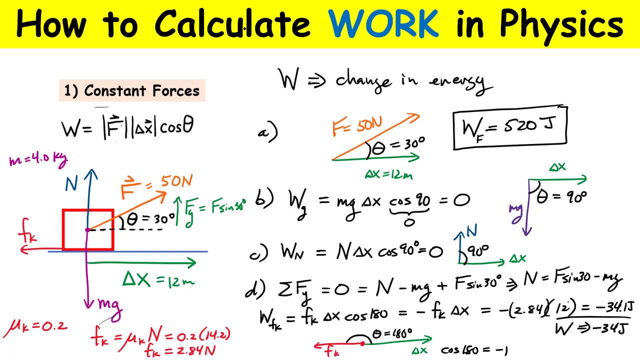 so I get minus 34 joules to be the work done by the force of kinetic friction. All right, so in this case we had two forces that actually do work. I had my applied force and then I had the work done by the force of friction. 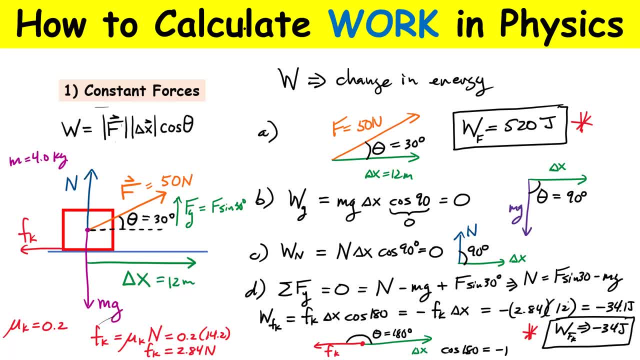 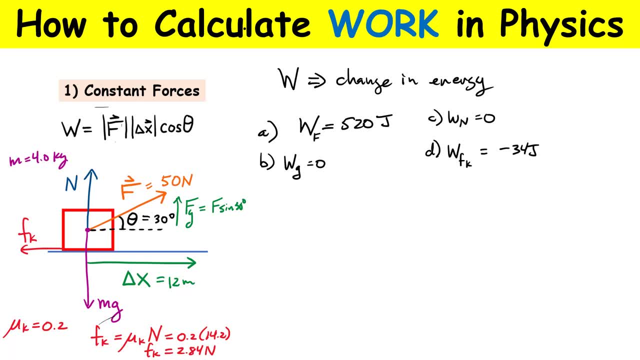 I didn't have any work done by these other forces, right? in this case They were both zero, So that's kind of interesting. All right, so if you put everything together, now again I go back to my definition of work. 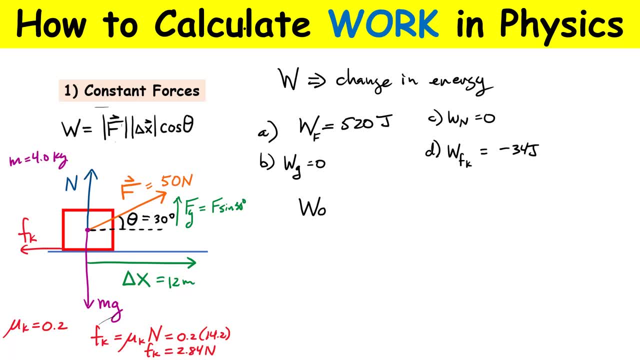 we can do something called the work-energy theorem. Okay, very important theorem in physics, And work-energy theorem simply says that if you calculate the net work on an object due to all the work done by the forces, okay, so in this case, here, if I would add up all of these quantities, 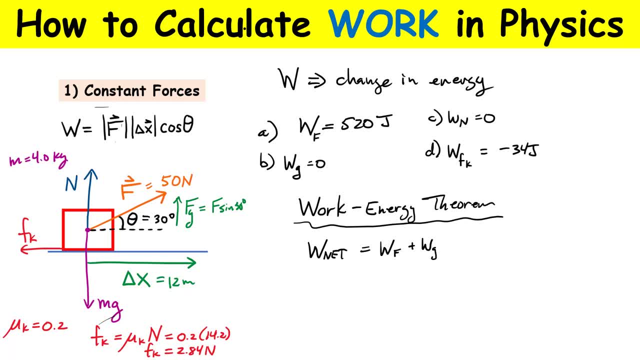 the work done by the force F, plus the work done by little g, plus the work done by the normal force, plus the work done by the force of kinetic friction. if I add all of those up, it has to be equal to a change in energy. 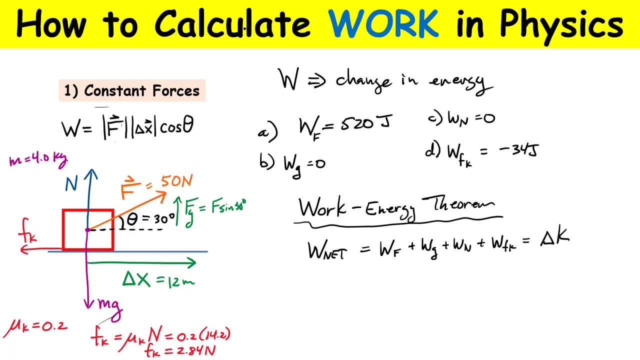 And it's a change in kinetic energy of the object. This is always a final value minus an initial value. So if we imagine here this block started initially at rest, so the initial velocity was zero meters per second, you might want to know how fast is it moving at the end, right. 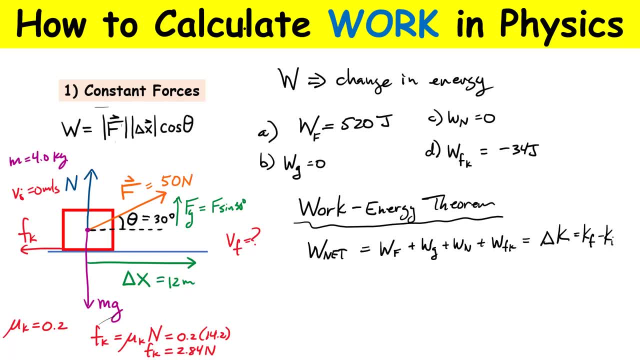 If I dragged it 12 meters and I did this amount of work. well, the work-energy theorem would be a useful theorem to be able to use to calculate that. All right, note that the initial kinetic energy would be zero because it started from rest. 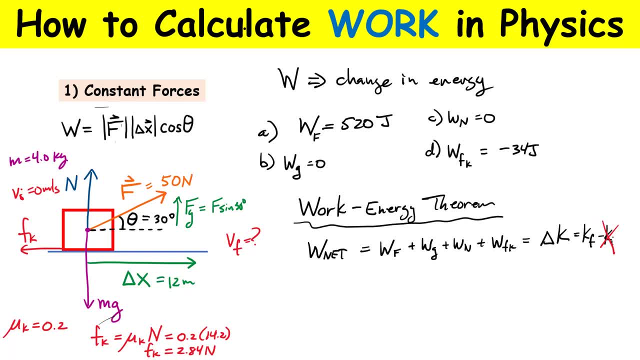 And now you add up all of these values right: 520 minus plus 34, that gives me 486 joules. That is the net amount of work done by all of the forces. That has to be equal to the final kinetic energy. 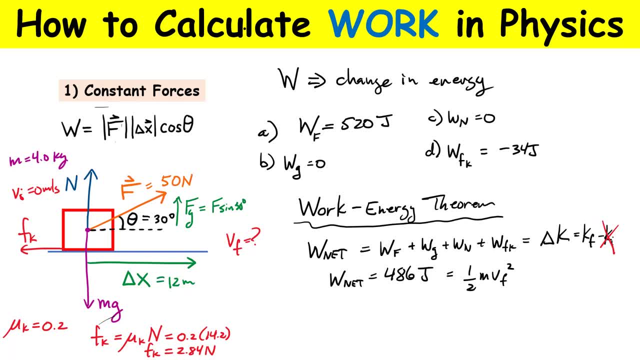 which is 1 half mv. final squared. Do a bit of algebra here. Bring this 2 to the top, divide by the mass and then take the square root. Your expression for the final velocity, or the final speed rather, would be 2,. 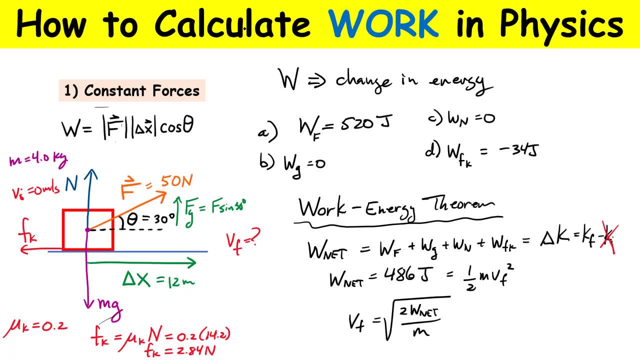 the net work divided by the mass of the object, which I told you was 4 kilograms. Now you substitute, in all the numbers, 2 times 486 over 4, rather, And that gives me approximately 15.6 meters per second. 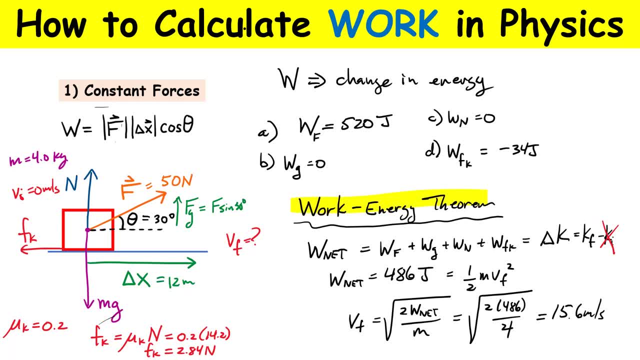 Okay, so that is a kind of an application of calculating the work and using it now to calculate other quantities, such as the final speed of an object. All right, here's another example dealing with constant forces. We have again a crate of mass m. 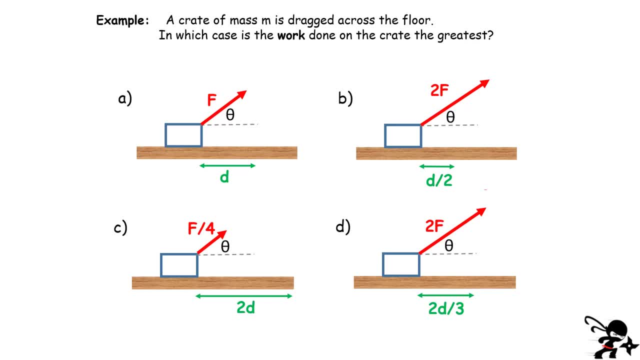 is dragged across the floor here, In which case is the work done on the crate the greatest, And we're looking at the work done by that force F right there. So I have four different cases where I'm giving you a force. Sometimes the force is bigger. 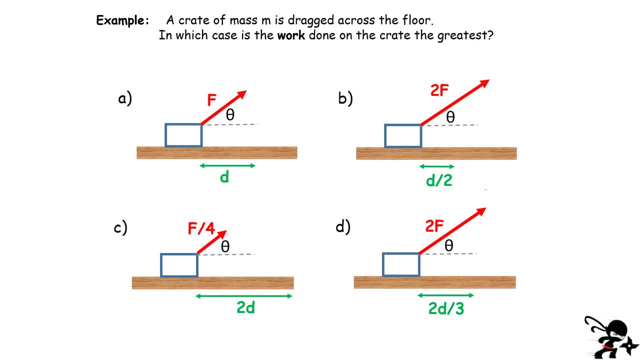 For example, this case is 2F. Case C has a smaller force: F over 4.. And sometimes the displacement is bigger or smaller, okay, depending on the scenario. So let's rank them from the greatest to the smallest. So we really have to calculate them for each case. 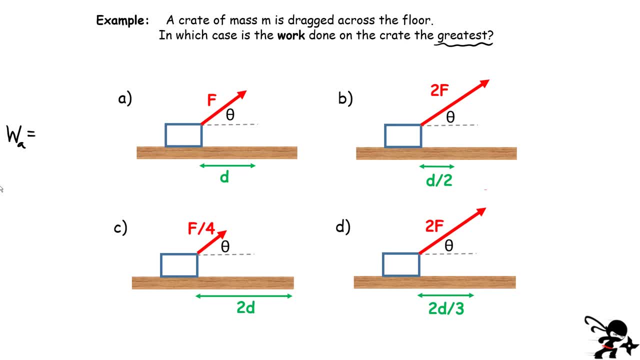 So how would that look like? for the first one, I'll just call it the work for case A. right, here I apply the definition. Remember, our definition was: what is the magnitude of the force? What is the magnitude of the displacement? Okay, multiplied by cos of the angle between them. 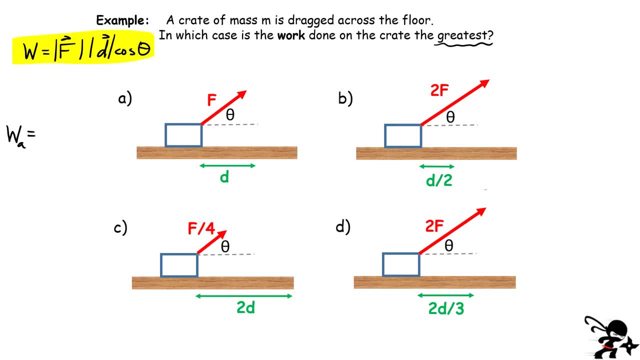 Since I have a constant force, you just apply that formula directly. So in this case, here we have a force F, We have a displacement D And I have cos of theta- The same thing as what this equation said. Well, let's have a look now at case B. 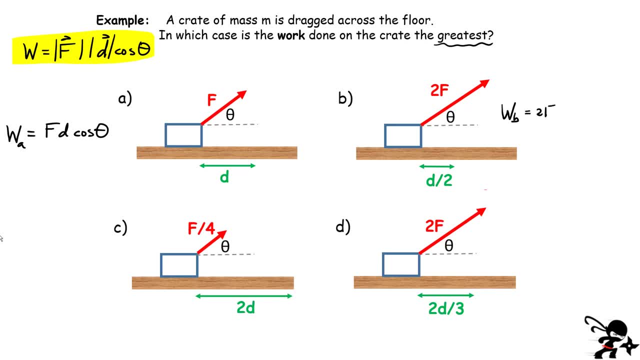 In case B I would have a force which is equal to 2F. in this case, Multiplied by a displacement is D over 2,. okay, because I'm only dragging it half the distance here, And multiplied I still have an angle here. 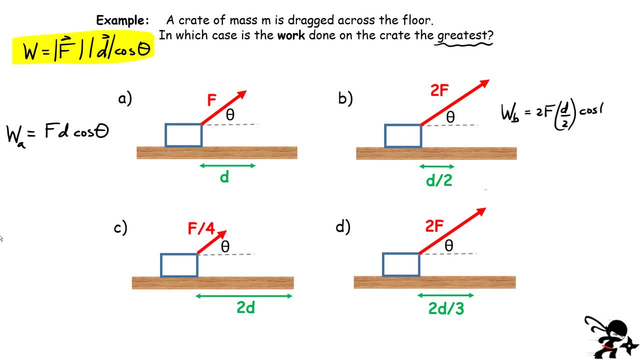 between the force and the displacement. Therefore, I still have cosine of theta. Now, if you simplify this a little bit, those twos will cancel out right. I have one in the numerator, one in the denominator. At the end I get the same answer for A and B. 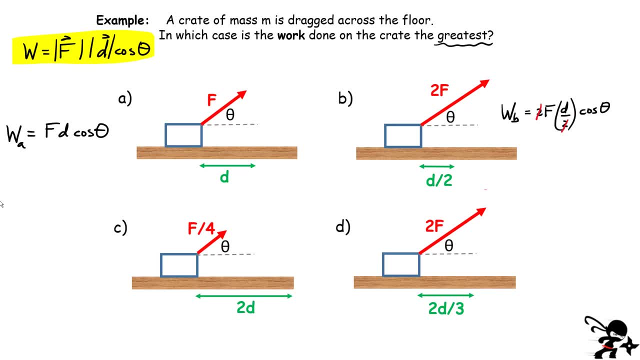 So it's the same amount of work done by both of those forces. How about case C? In case C we have magnitude of the force F over 4.. Magnitude of the displacement: 2D. Again, cosine of the angle theta. 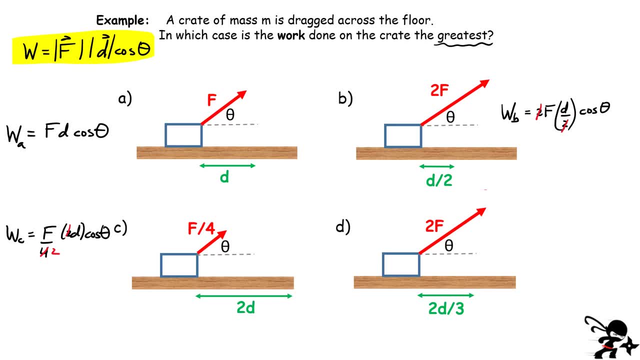 Cancel out a 2 here, Factor out a 2 here And look what we have here. We have FD, cosine theta, And I still have a 2 left over here. I'll just go divide it by 2.. That is the work done by this force for case C. 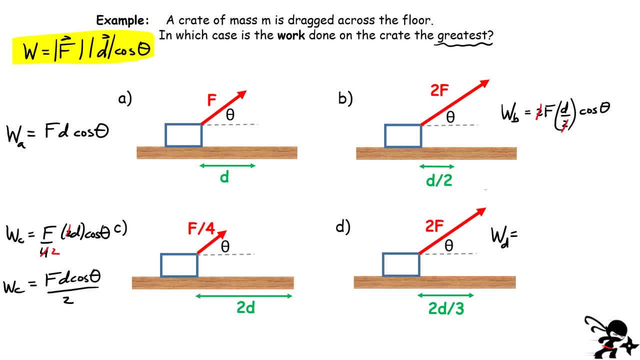 And our last one over here, this one here: the work done in case D would be the magnitude of the force, 2F the magnitude of the displacement. In this case it's 2D over 3.. Okay, and now multiplied by cosine of the angle, theta. 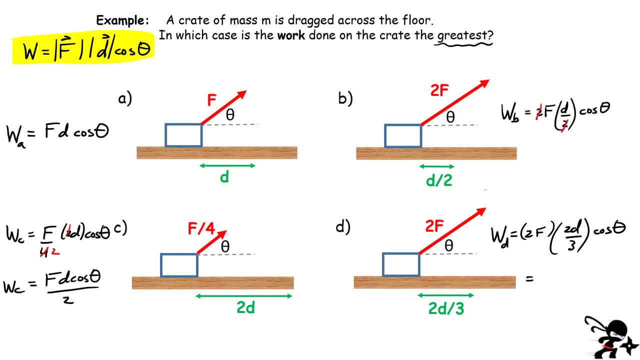 All right, let's group together all the number terms. Okay, so we have 2 multiplied by 2.. We have 4 thirds here. That pops up in the front, And then I have FD, cosine of theta. Okay, and that's the work done for case D. 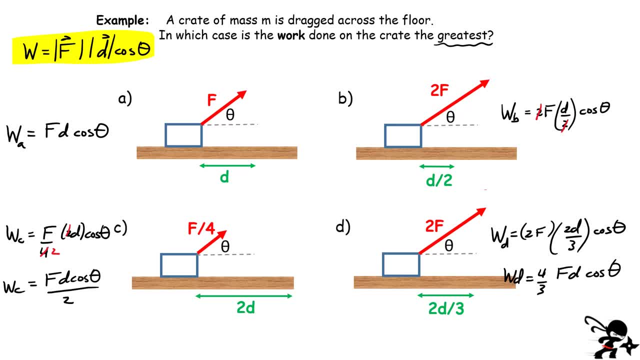 All right, let's compare. So 4 thirds is bigger than 1.. So this is how they would be. I would have the work done in case D is the biggest right, And then what would you have? You'd have A and B that are equal to each other. 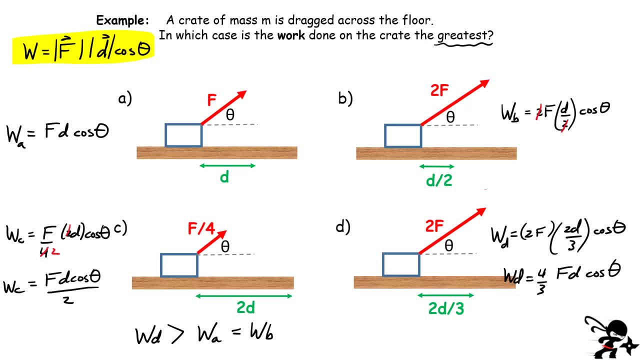 So I would write: A equals to the work done in case B, And then that's bigger. The smallest one is actually this force over here for case C. So that's how I would write that answer, going from the greatest to the smallest. 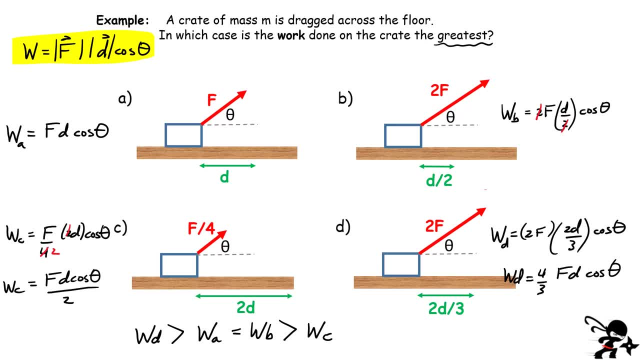 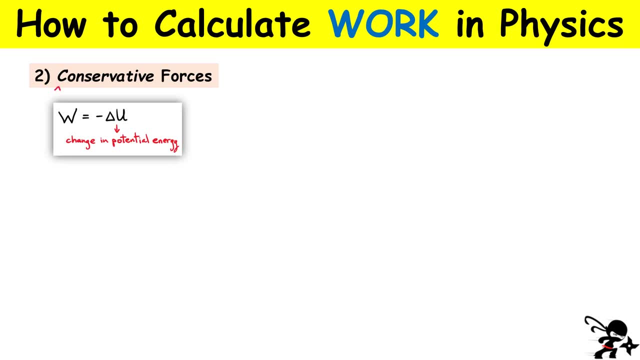 Okay, kind of a nice example for constant forces. All right, and now I want to calculate the work using a different method, And the method that I'm going to describe here can be applied to conservative forces. So, conservative forces, let's maybe just think about some examples. 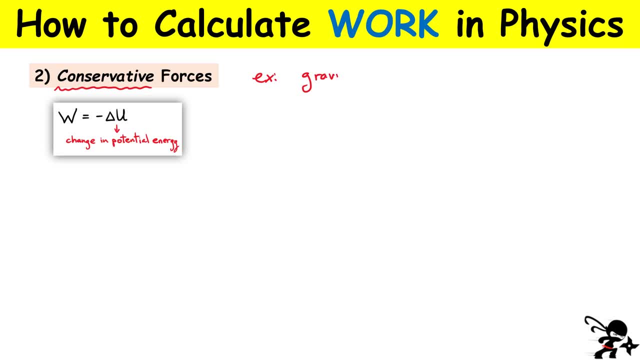 of some conservative forces. So the force of gravity is a conservative force, also from an ideal circle. So a spring: okay, That force is a conservative force. And you might later see like electrical forces: okay, forces between charges, Those are conservative forces. 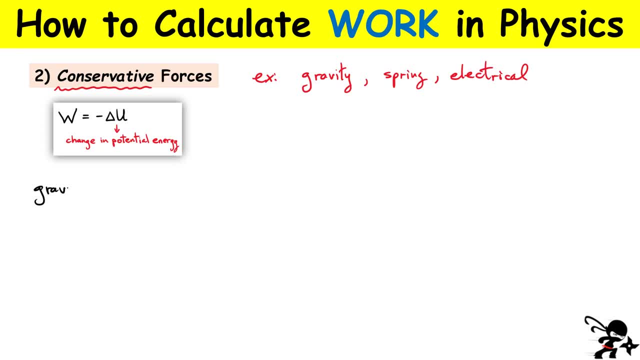 So let's consider gravity, for example. Okay, so if you consider the force of gravity, and for now let's just consider an object close to the Earth, all right, We have an object here of mass m. There is a force of gravity, all right? 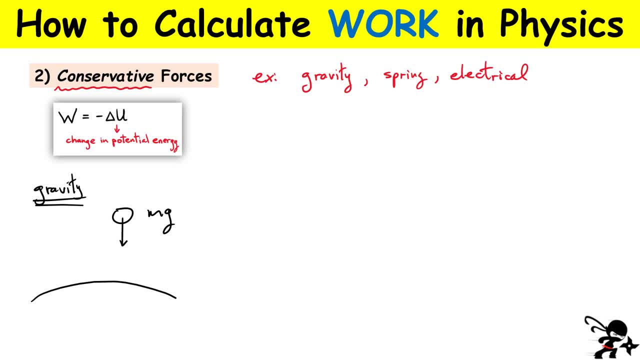 The Earth is pulling down on that And the force is simply mg. right, That's the weight of the object. Okay, For a spring force? let's go ahead and write this: For a spring force. you imagine we have an ideal spring. 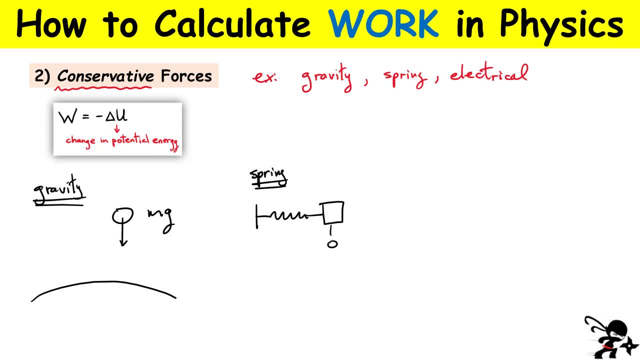 and there is a mass m attached to it. It's initially at some position and then we decide to stretch it. all right, We stretch it a certain distance, x. Okay, now we have to apply a force in order to stretch it. 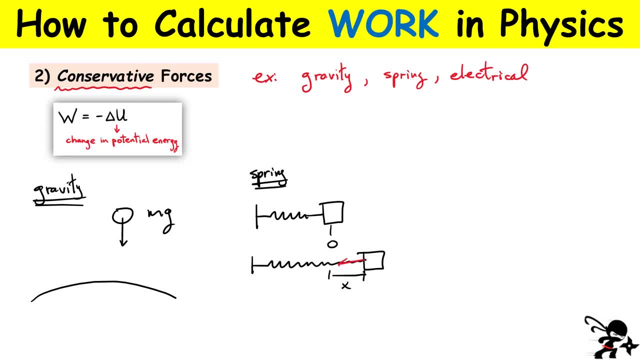 But once it's stretched there, the spring wants to bring the mass back and the value of that force is given by Hooke's Law. It's given by minus kx. k is a property of the spring. okay, It tells you how hard it is to stretch or compress it. 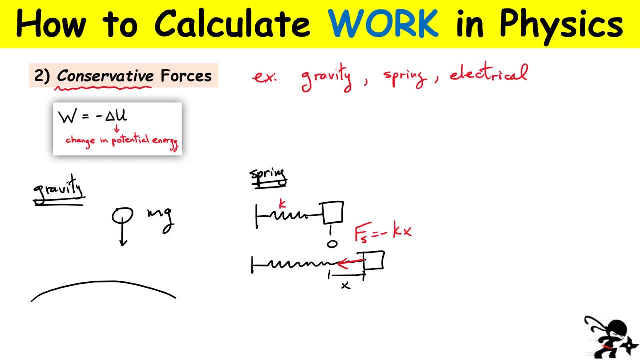 And x is the amount of distance that was stretched or compressed. okay, This is an example of a conservative force. Now the other example would be an electrical force. okay, Later on in your class you might see electrical forces, The force between two charges. 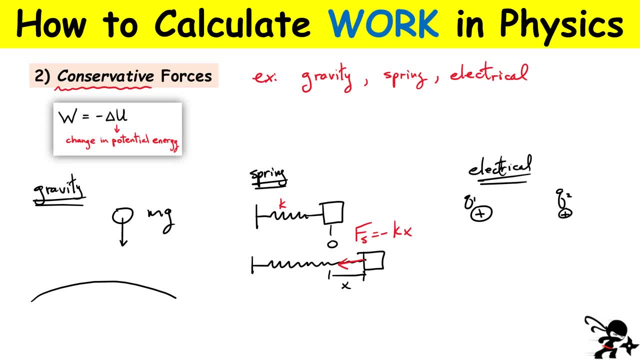 q1 and q2, is given by something called Coulomb's Law. Coulomb's Law can be written as this: kq1q2 over r squared. okay, That is the force between both of those charges, If both charges are positive. 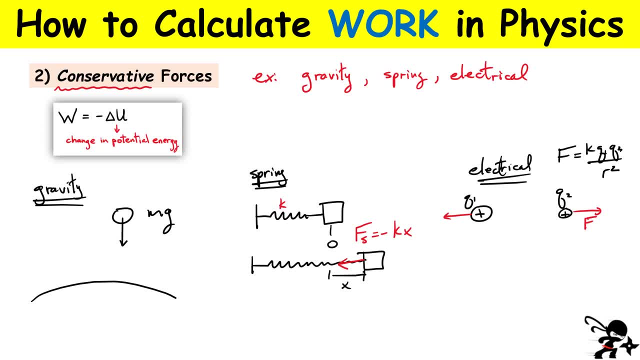 then there would be a repulsive force. for example, given like this: okay, These are three conservative forces. Now, whenever you have a conservative force, there is always a potential energy associated with it. Okay, we always can define a potential energy u. 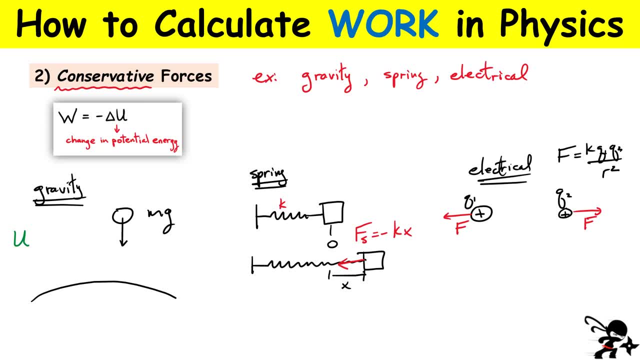 related to this system. okay, For example, for gravity, you might see that the potential energy is given by mg multiplied by the height. okay, And the height here would simply be this value here. So we'd say there's zero potential energy. 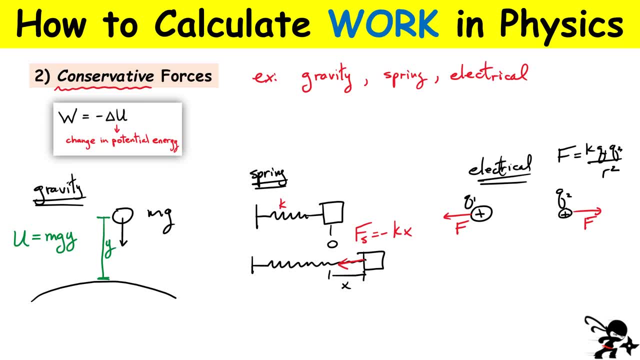 when that mass is near the surface of the Earth, And then I have to apply a force in order to bring this mass a certain height. So I've stored some gravitational potential energy in the system. I'll just call that u with a little g there. 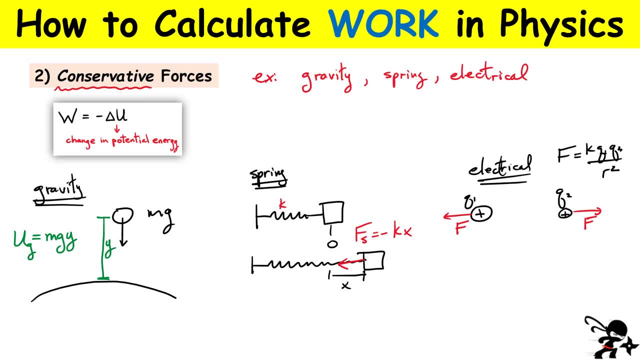 For the spring. it's the same thing. For me to move this mass, I have to apply a force, and then there's a spring force acting opposite of that. But there is a potential energy now. There's energy stored in this spring mass system. 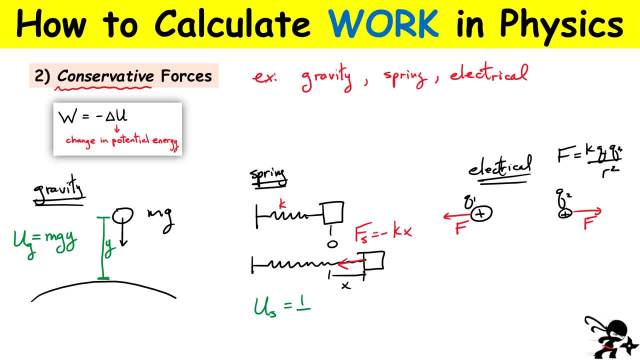 And that potential energy for a spring mass system is given by this 1 half kx squared. All right. and the last one here would be well, these two charges For me, for example, if they started initially very close to each other. 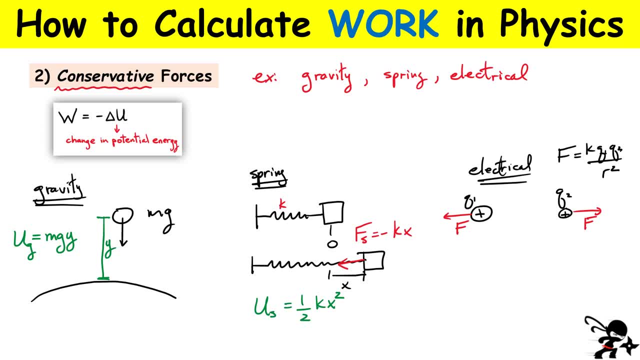 and then I wanted to separate them. right, you might apply a force in order to separate charges. There is again a potential energy associated to the charge system. okay, And for electrical charges, again, I'll just call that electrical potential energy. 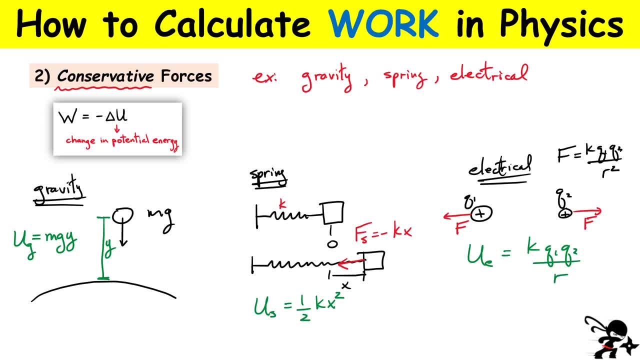 and it would be given by this value here: kq1q2 over r. So that's how you know it's a conservative force, And the nice thing about conservative forces is you can always calculate the work done by a conservative force using this equation. 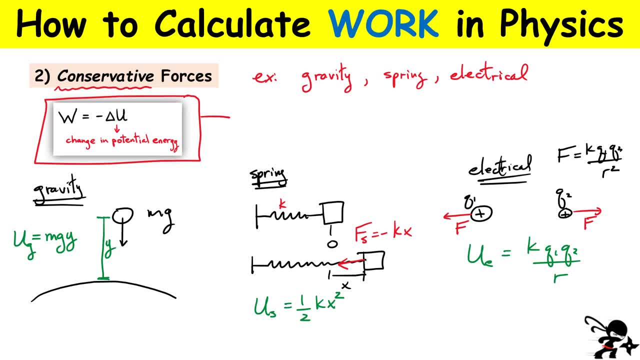 Okay, now what does this equation say? It says that the work done by that conservative force- so it's either gravity, spring, electrical, those are examples- is given by this minus the change in potential energy. So it's minus. what is the change? 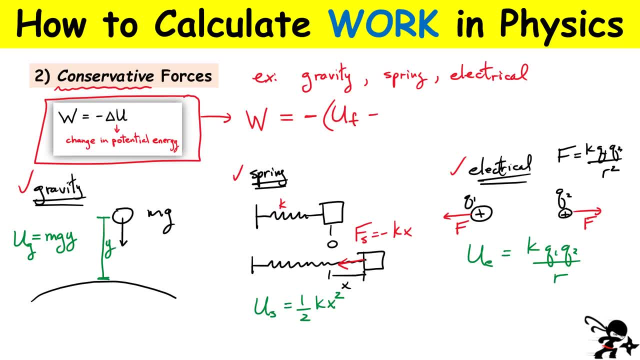 It's always a final value of potential energy minus an initial value of potential energy. Now if I distribute this negative sign here throughout, what you end up getting then is I'll just switch the order here so I get the initial potential energy of the system. 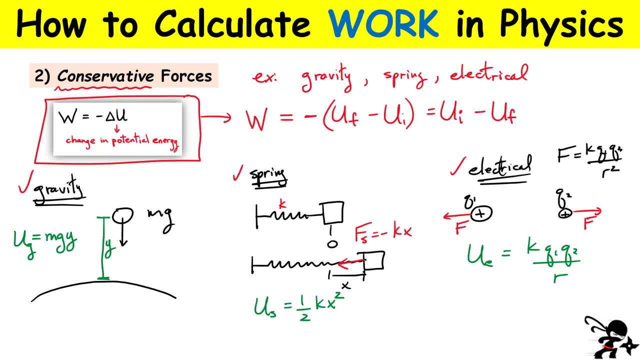 minus the final potential energy of the system. All right, this is the equation that you can use now to calculate the work done by that force, that conservative force. One thing we notice about this is that it only depends on two things: What is the initial value and what is the final value? 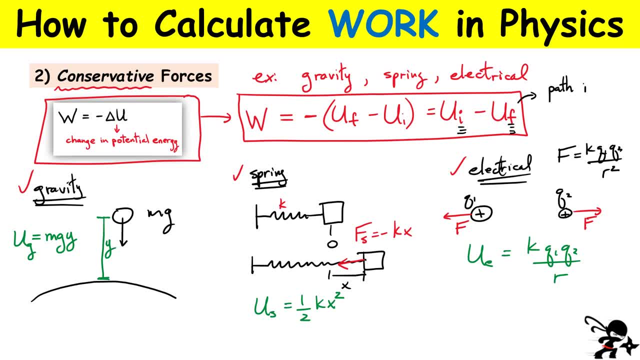 Okay, we also say that it is path independent. It doesn't matter how you actually got there right. It didn't matter on which path that you took. It only depends on what was the initial value of the potential energy and also what is the final. 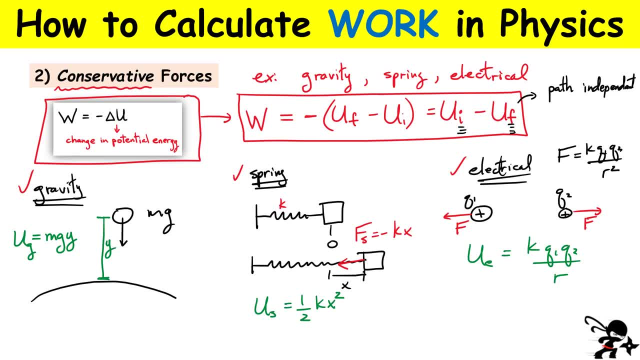 Intermediate values do not matter. That is also a definition of a conservative force. So one thing, let's just highlight some examples of non-conservative forces. okay, Non-conservative forces, oh boy, I'm having trouble spelling today. Let me just get that right. 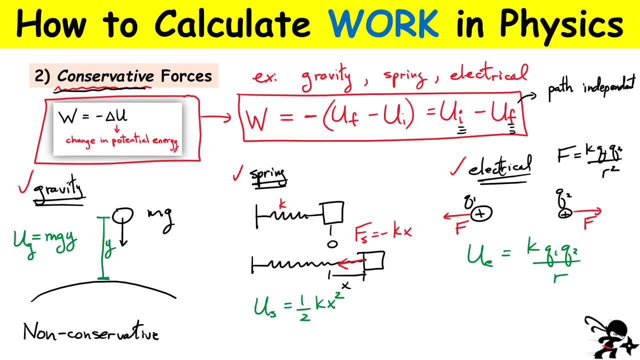 Non-conservative would be, for example, the force of friction, right, Anything that has any kind of dissipation, for example drag right, The motion of an object through a fluid like air. right, There might be this resistive force called drag. 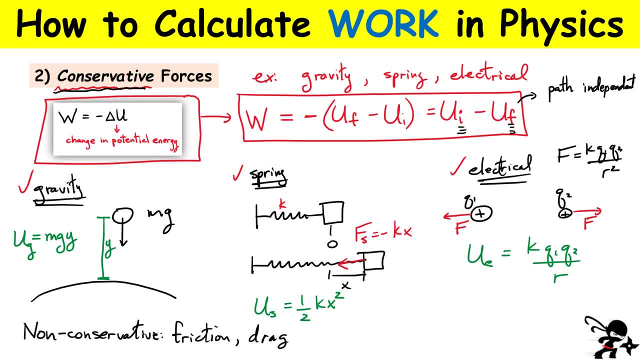 In those cases here you can't define a potential energy, okay, It doesn't make sense for this case, because in those cases the work done by these forces, okay, they actually not only depend on the initial and the final, but they're also path dependent. okay. 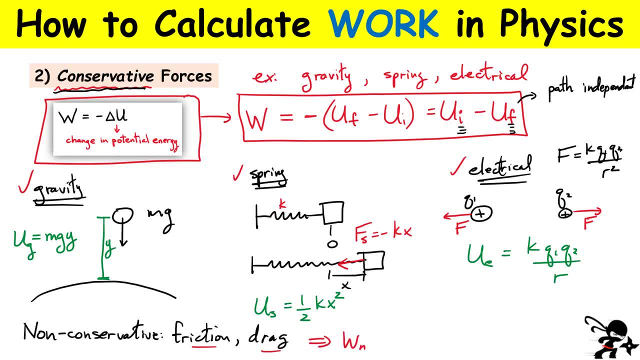 So in order for you to calculate the work done by a non-conservative forces, you'd have to consider the entire path that you're taking. okay, So path dependent. All right, let's go back and examine this formula and use an example problem to see how we can calculate it. 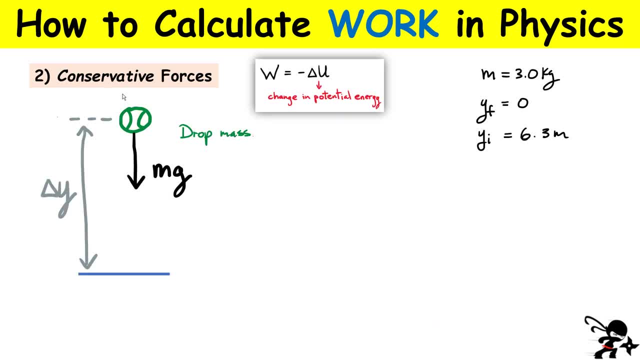 All right, let's consider this simple system here. I have a ball up here. Let's say it's a heavy one. The mass is three kilograms. It starts from this initial height. up here, The initial height is 6.3 meters. okay. 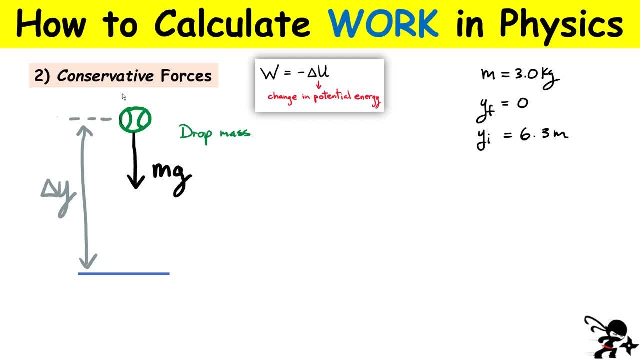 above the ground, okay, And I end up just kind of releasing that- and the force of gravity is acting on it. It's going to end up being right down here, Here near the surface, okay. So this is kind of the final position. 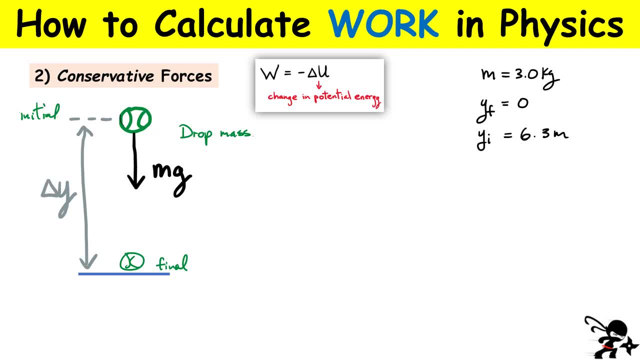 The initial position was up here at the top. Now we want to find what is the work done by gravity? okay, By the force of gravity. I'll just call it the work done by little g. Now I want to use, since I know that gravity. 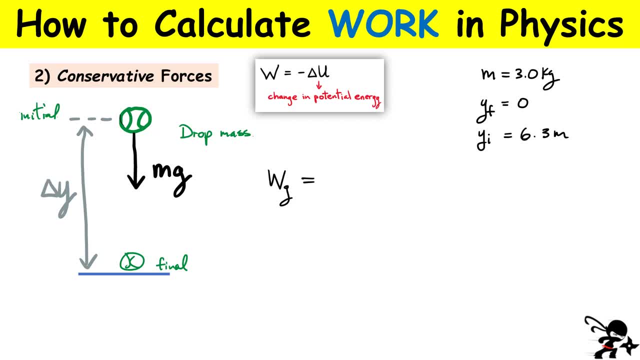 is a conservative force. I can use my minus delta u. So I would simply do minus u final, minus u initial, okay, And again, you can distribute that so you get the initial minus the final, So the work done by gravity. Now what is the initial potential energy of the system? okay, 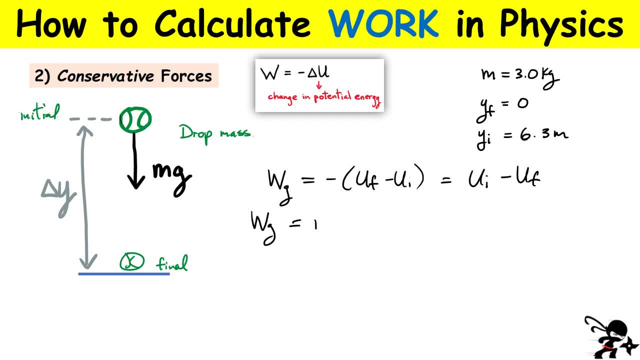 The initial potential energy is when I'm at this initial position. So again, it's mass times, little g, multiplied by that initial height and minus the final gravitational potential energy, mg, multiplied by my final height. okay, So now you just substitute our values. 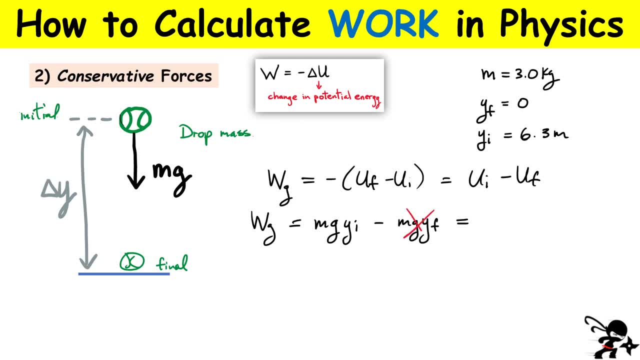 First of all, we know that the final position is zero, so there is no gravitational potential energy over here, And initially, all I have then is: the mass is three little g is 9.8, and the initial height was 6.3 meters. 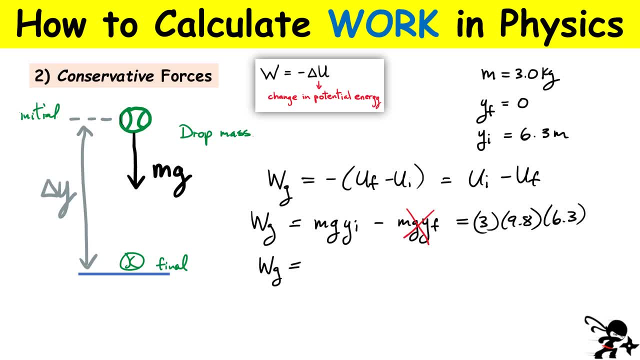 Notice that I get. the work done by gravity is going to be a positive value in this case, right? And if you substitute the numbers, you should get 185.2 joules. okay, Now think about it. Why is it positive, right? 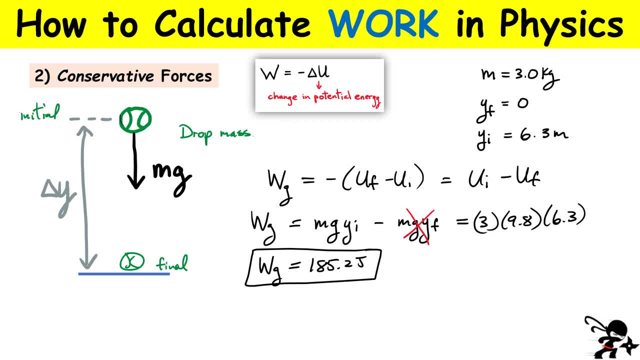 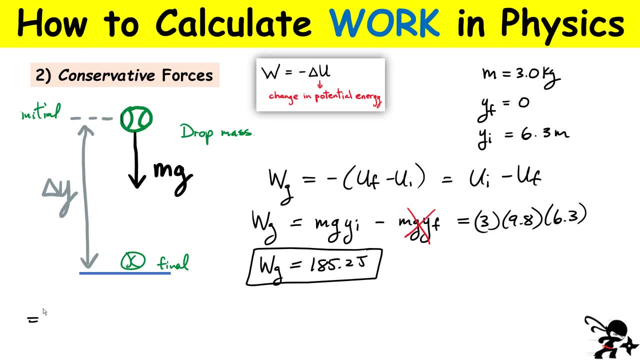 Well, if you go back to kind of the first types of problems where we dealt with constant forces, this is a constant force, which means that I could also calculate the work done by gravity. I'll just call it work done by little g, using the first equation that I had right. 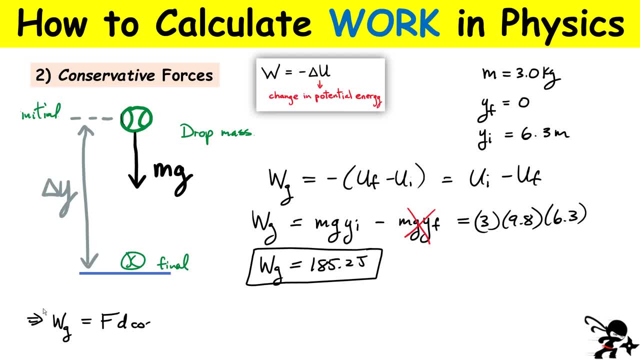 I have a force. I have a displacement multiplied by cos of the angle between both of those. So let's just think about it. You have your force here, which is mg acting down What else? Well, yeah, I also have my displacement. 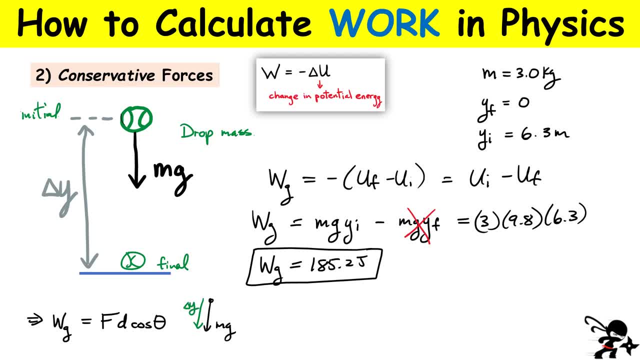 which is also acting down, and it has a value: delta, y And the angle between both of those. again, this has to be the angle of 0 degrees. Both vectors are parallel to each other, So you go ahead and you substitute my values here. 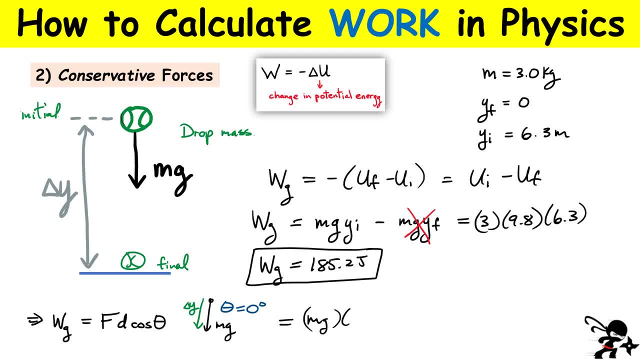 for the force. The magnitude is mg, The displacement is delta, y and then cosine of 0 degrees. Guess what you have? You have this exact same equation right: 3 times 9.8 times the displacement magnitude, 6.3,. 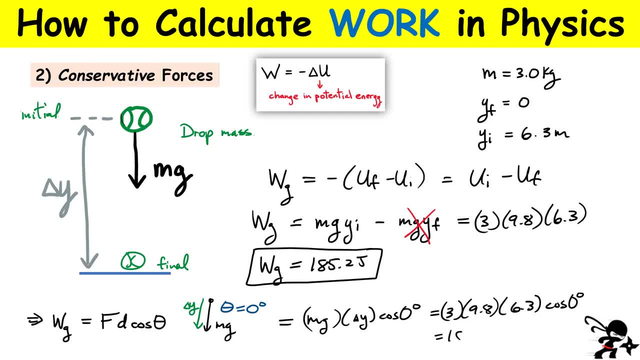 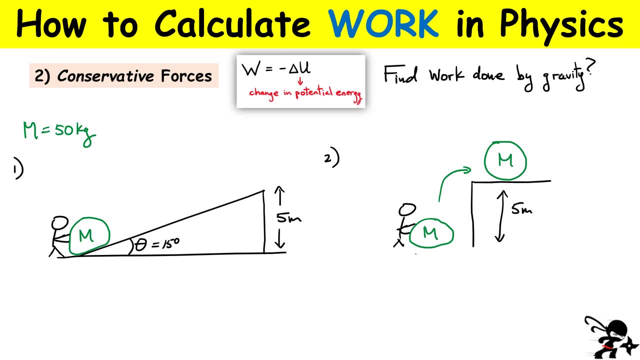 and again cosine of 0. All right, So you get 185.2 joules using the constant force equation for work. Okay, Pretty straightforward, All right, Consider this simple example over here. So you have this kind of heavy mass of 50 kilograms. 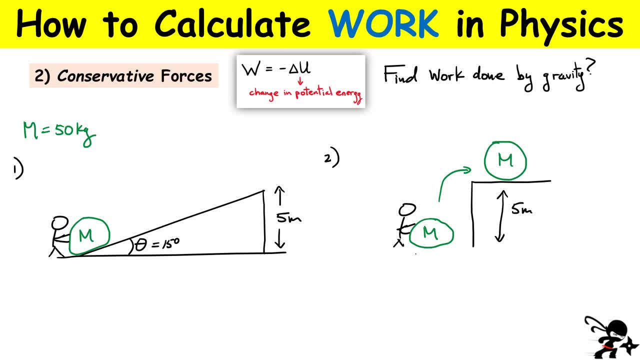 and you have two cases. My goal is to get it at the top of this 5-meter hill, All right. So in case number one, I can either push it right up the ramp- here The ramp makes an angle of 15 degrees. 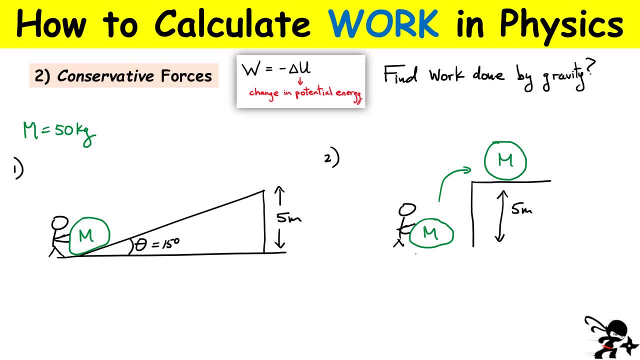 with respect to the ground And I want to get it all the way to the top. In case number two, I'm just going to kind of lift it and place it at the top, or I can just throw it, if I can. Okay. 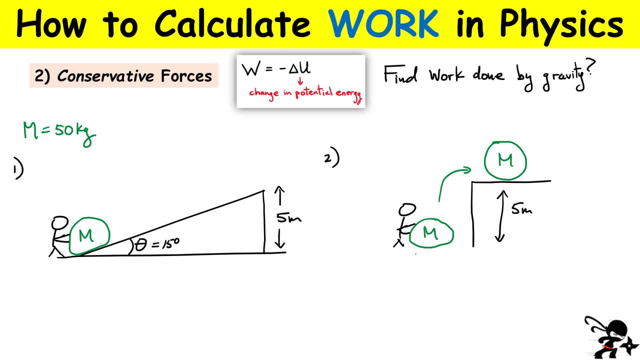 So what if the question was: find the work done by gravity? Okay, Well, gravity is a conservative force, so you can use this equation here. It's minus the change in potential energy, which we said was equal to initial, minus my final gravitational potential energy. 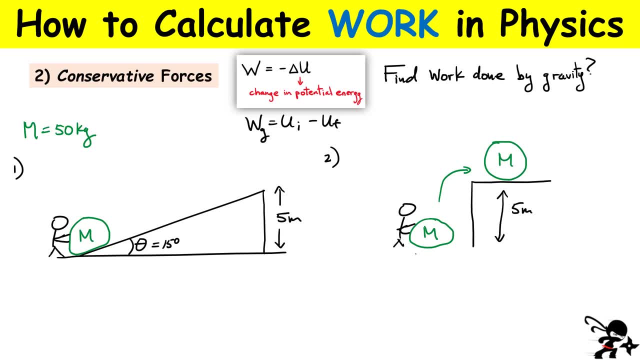 since we're looking at the work done by the force of gravity. Now again, if I set, U equals to zero on the ground for both cases, that means initially I don't have to worry about it. I have zero potential energy in both of those cases. 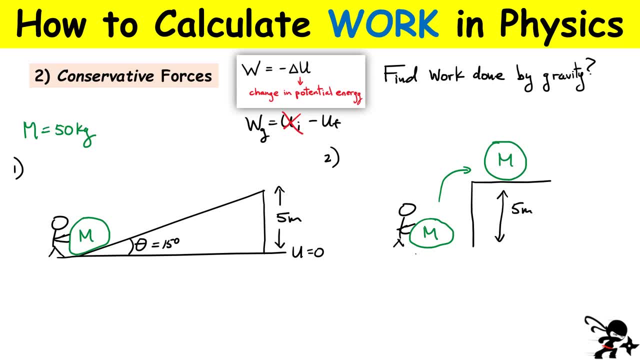 All I need to calculate now is what is the final potential energy. Again, potential energy is given by Mg multiplied by the height, And in this case it would be the final height. So the work done by gravity in this case here would be minus Mgy. final. 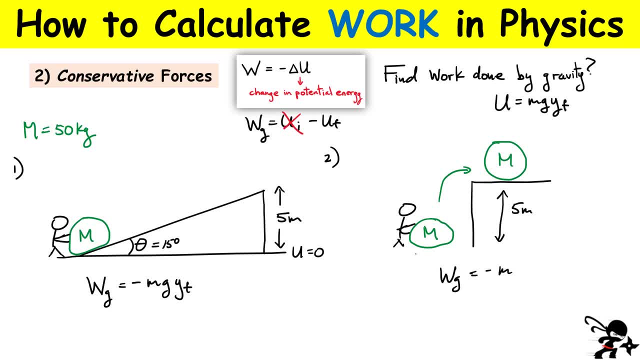 Okay, And in this case, here would be Wg would be minus Mgy, final. Now you see, in both of these cases the final height is this one, right, And it didn't matter how I got there. in both cases it's five meters. 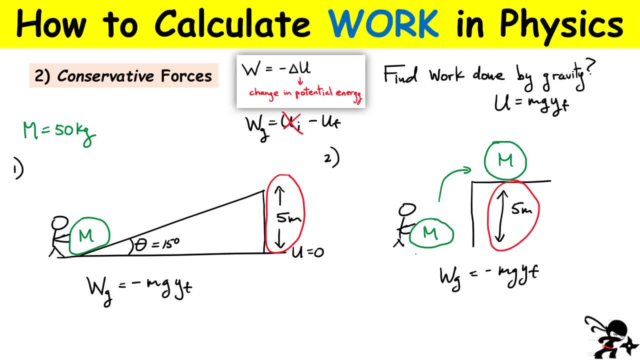 So they have to be the same, Although the path is considerably different. right, This path is probably much longer than this one. This one's just going straight up. It's five meters. This one's going to be this whole length of this ramp. 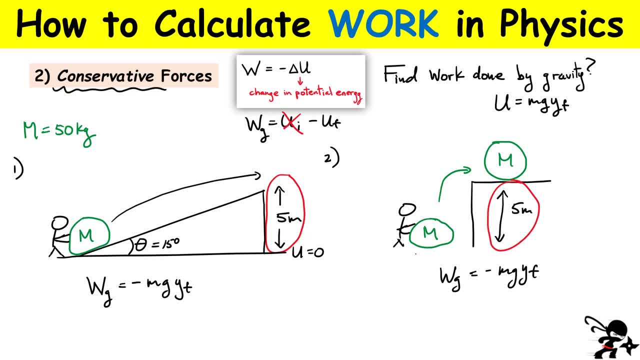 That's because we're dealing with a conservative force and it is path independent. So at the end we just substitute our numbers. So we get minus 50.. We get 9.8.. And my final height was five meters. I put that in a calculator. 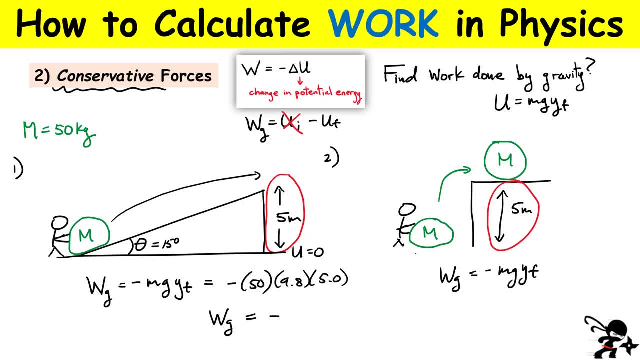 and I get, the work done by gravity is a negative number in this case, And it's 24,000.. 2450.. Okay, Now why is the work done by gravity a negative value? Well, again, if you think about it, in this case, 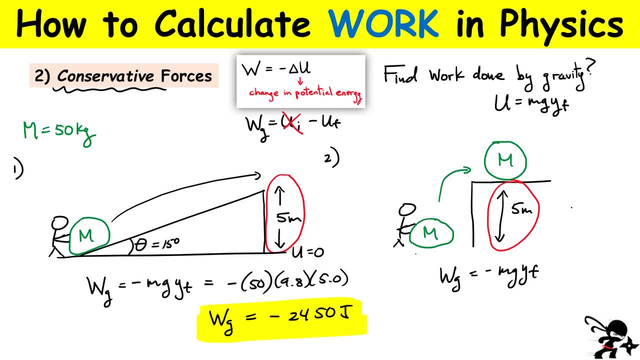 what do we have? right? We have a displacement which is going up, right, That's my displacement, Delta Y, And the force of gravity during this is down, Okay, Whenever you have a force that is in the opposite direction of the displacement. 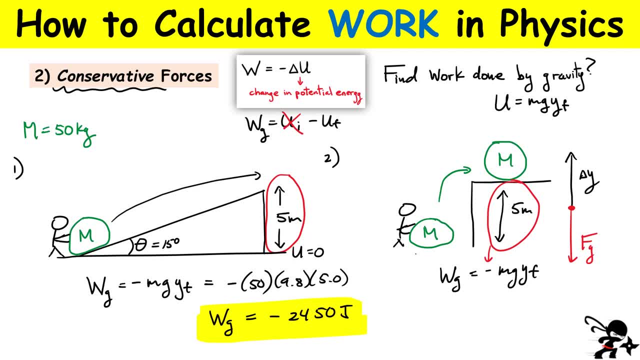 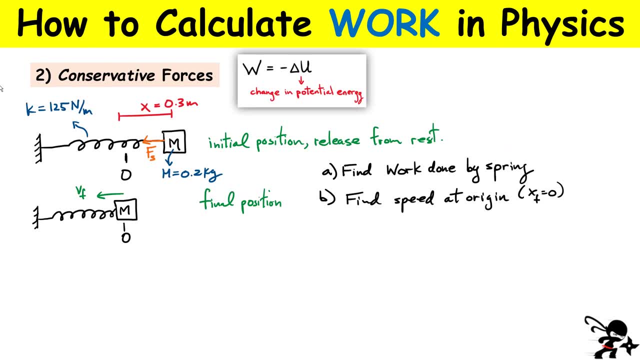 guess what? You're going to have negative work done by that force. Okay, So don't worry about that. All right, Let's do another case with conservative forces. but let's consider a spring problem now. Remember for a spring. the potential energy stored in a spring is equal to one half KX squared. 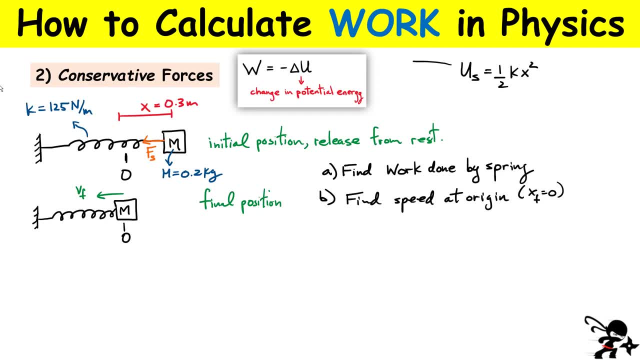 And again, if this is a conservative force, the easiest way I can do to calculate the work is to use my equation here. Work is negative, the change in potential energy of the spring. All right, So we're going to consider this situation here, where I have a block of mass M. 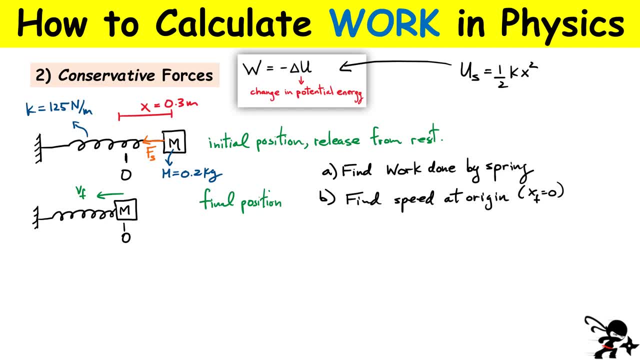 which is 0.2 kilograms, And it's initially stretched out a distance of 0.3 meters, And here it's released from rest. Okay, So that's kind of the key. Okay, So now there's a force acting on it. 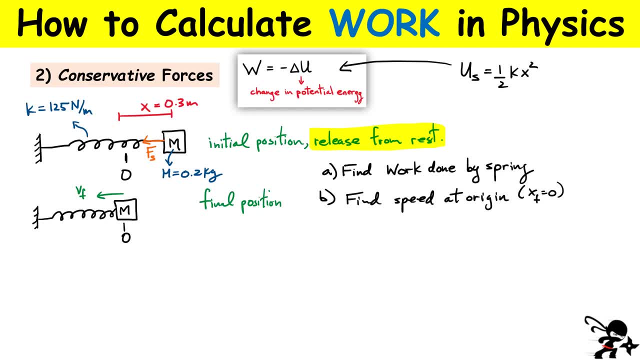 Hook's law tells me there's a force of the spring on this mass and it's pulling it toward this equilibrium position, So it's going to start to speed up. As it speeds up, it gains kinetic energy right, It gains more speed. 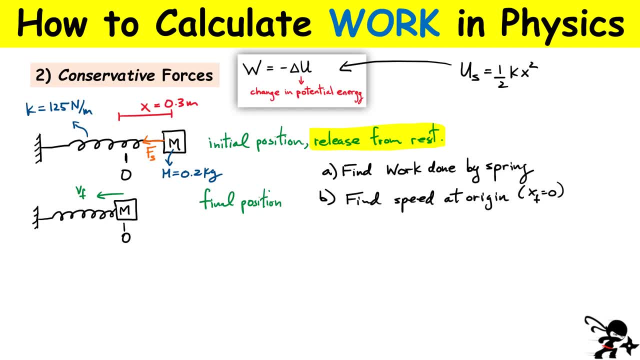 Okay, And I want to know in the second part, how fast is it moving once it crosses this origin right here? All right, So the first part is find the work done by the spring. Okay, So that one is pretty straightforward, right. 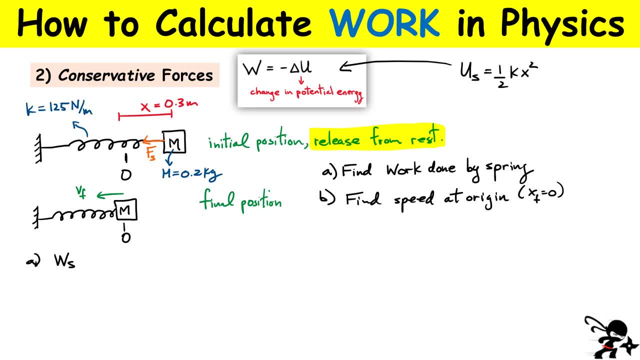 You simply write the work done by the spring. Now, it's not a constant force, So be very, very careful. right, Not constant. So if you were going to try to use the work is F: D cosine of theta of zero to cosine of zero degrees. 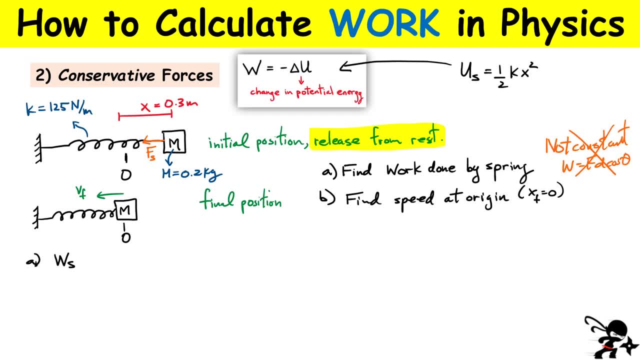 uh, you'll unfortunately get the wrong answer because the force changes as the spring decompresses. right, The force is a function of how far you stretch it, So it's not a constant value, All right, But we can use this equation, right here? 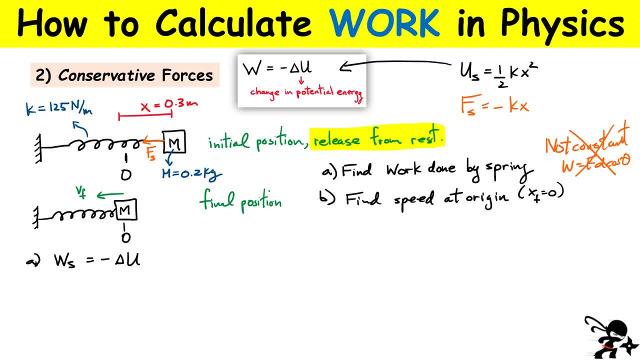 So the work done by the spring is minus the change in potential energy of the spring, So it's minus. this is a U final minus a U initial. distribute that negative sign through So you get the initial potential energy in the spring minus the final potential energy. 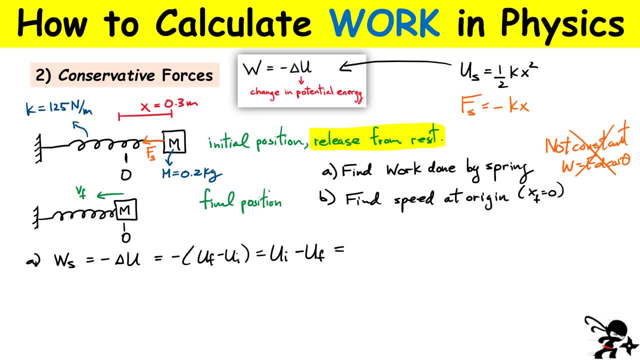 In the spring. So now we use our definition of potential energy. So I have one half the spring constant K multiplied by my initial amount of stretching that I have minus one half K, X, final squared: All right. So there is a simplification here that happens. 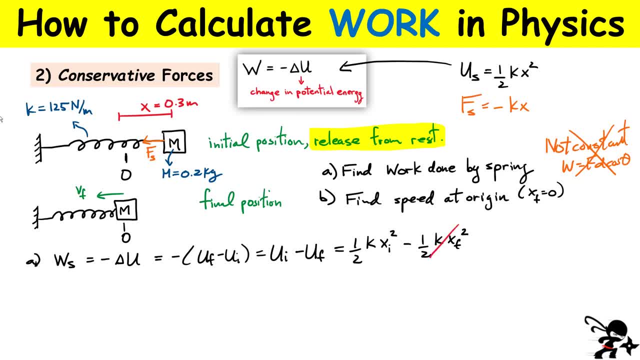 My final position is what I'm when X equals to zero. So I don't have to worry about this term, right Cause I substitute: X equals to zero, right there. And the initial value I can just substitute. in all the numbers I have one half. 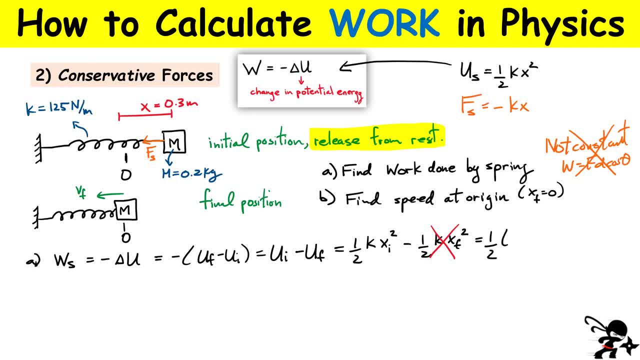 My spring constant for this spring is 125 Newtons per meter And the amount of initial amount of stretching that I had was 0.3 meters. I have to square that value. All right, You substitute the numbers in the calculator and you should get a 5.625 Joules. 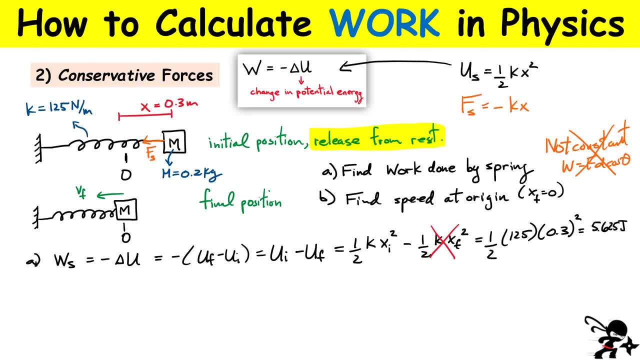 Okay, So that's the amount of work done by the spring. Let me just rewrite it over here: 5.625 Joules. Now it doesn't make sense to you that it is a positive value. Well, it should be right, because if you think about it, 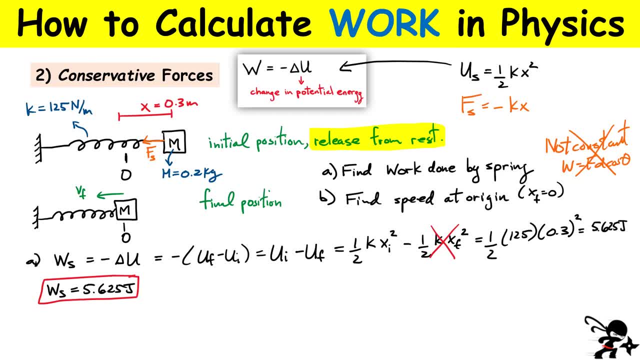 what do we have? We have a force acting to the left, right. Although the force is not constant, it's still acting to the left and my displacement right. It's still in the same direction: right, And the force is that way. 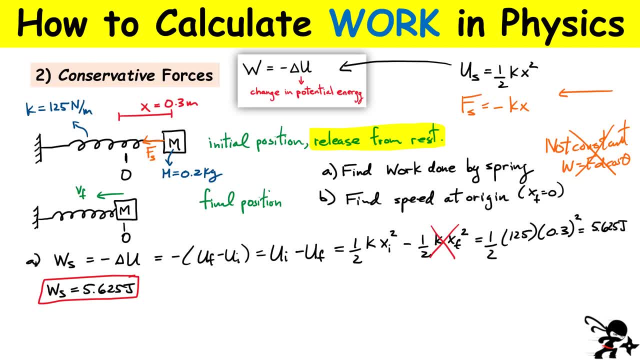 Whenever you have this situation, you're going to have positive work done by that force. All right, The next thing is to make sure that you're not just making it up. You're making it up, You're making it up, You're making it up. 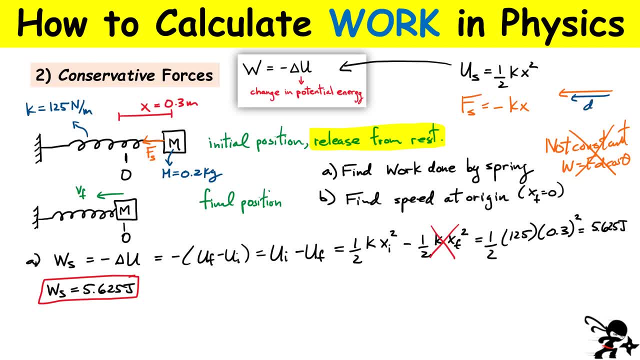 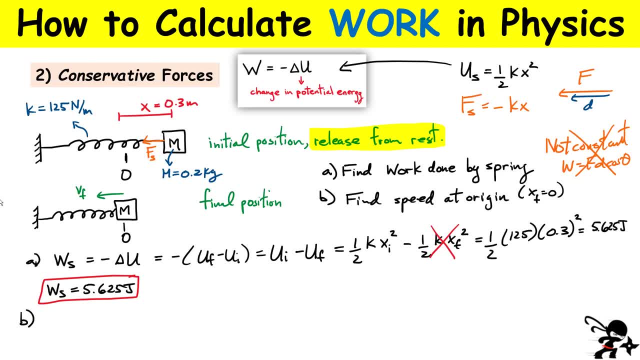 So for this, for part B, what I'm doing now is I'm going to apply the work energy theorem. So think about this mass M. Let's list all the forces acting on it. as it's moving, You have that spring force. 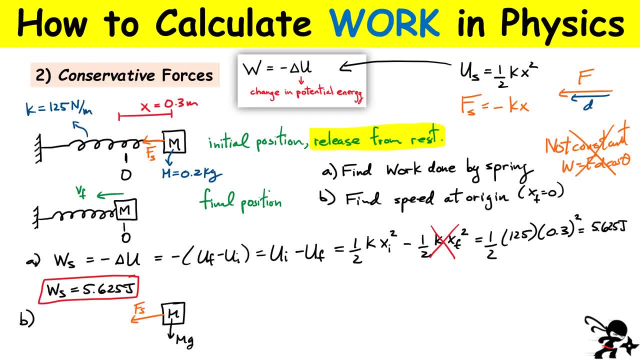 I have the weight acting down right MG, And I also have a normal force, and just forget about friction for now. All right, The problem is simple as possible. So if I want to apply the work energy theorem, work energy theorem says the net work done. 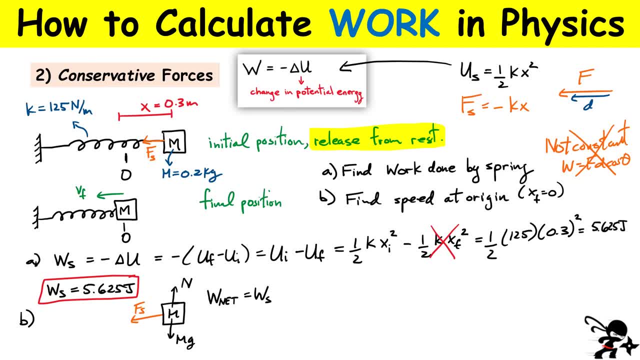 by all of these forces. that's the work done by the spring plus the work done by gravity, plus the work done by normal. If I sum all of those together, that has to be equal to the change in kinetic energy. And this is 1 1⁄2 mv final squared. 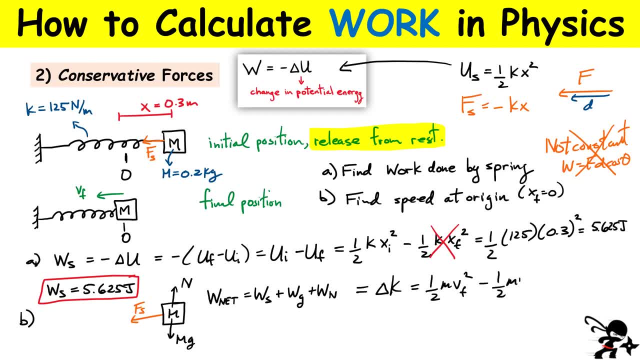 that's the final kinetic energy minus 1 1⁄2 mv initial squared. So if I release the object from rest, there is no initial kinetic energy. right, here And now there are some simplifications also right. The work done by gravity in this case also must be zero. 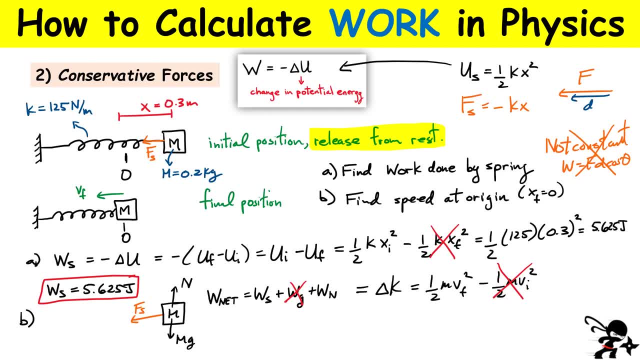 because gravity is acting down and the displacement is to the left. The work done by the normal in this case is also zero, again, because the angle between the force and the displacement is 90. So the only thing we're left with is what we just calculated in the first part. 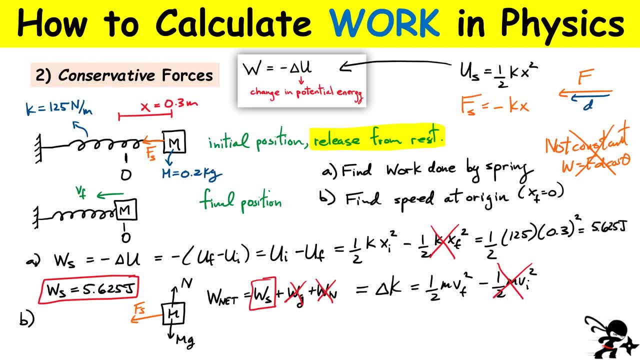 All right. so the last thing we want to do, then, is simply solve what is the final speed of this block as it rushes through this equilibrium position. So I have my equation right here. I'm going to bring the two on the other side. 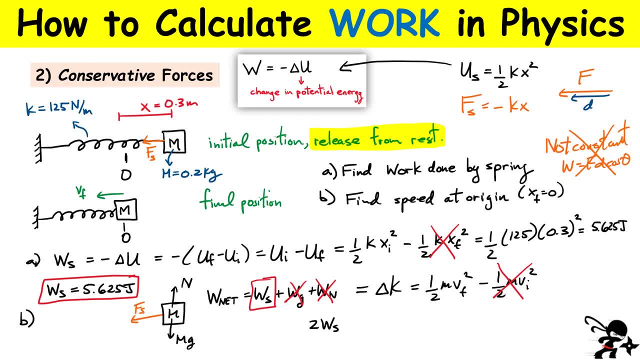 I have two multiplied by this work done by the spring. Now I have to divide by the mass That equals to vf squared, And to eliminate that I have to divide by the mass Now that equals to vf squared. So to eliminate the square. 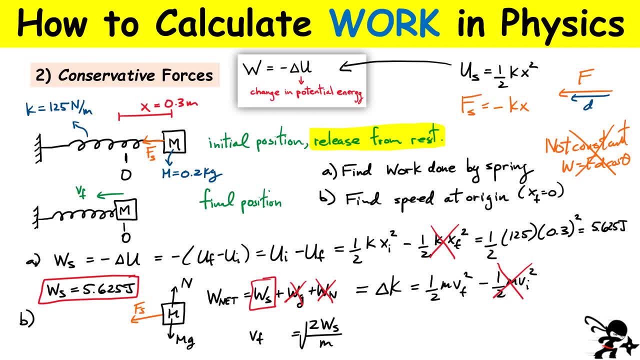 what you do is you just take the square root of both sides And now we substitute in all our numbers, So I get two The work done by the spring, I obtained 5.625 joules. Now the mass was 0.2 kilograms. 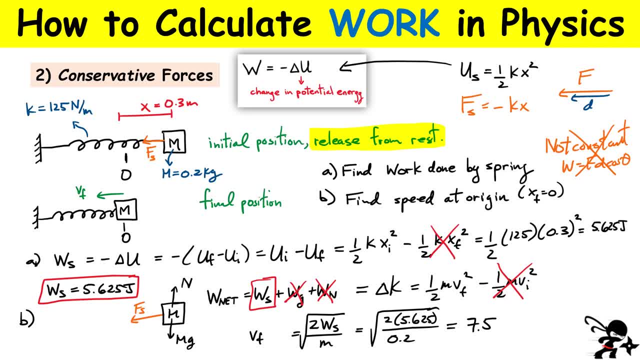 All right. if I put everything in the calculator and did things correctly, I should get 7.5 meters per second. So this is an application again of our work energy theorem. It allows us to calculate the speed Once we've calculated the work. 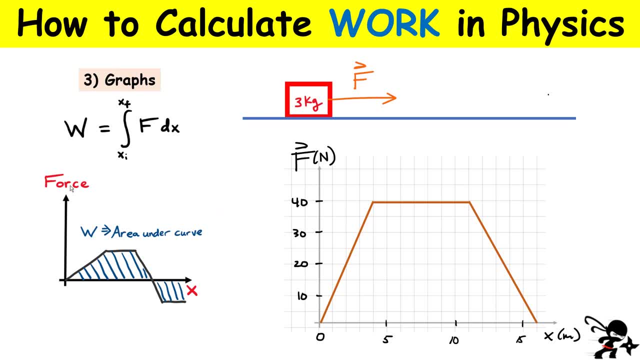 All right then. the third example I want to do is sometimes you're given a graph. You're given a graph of force and position of an object And it may have some line here which describes a force, And again it doesn't have to be a constant force. 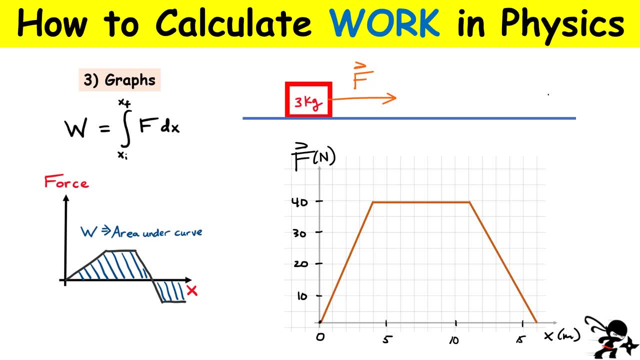 In this case the force starts at zero and then goes all the way to 40 Newtons, And then it stays constant for a while at 40 and then it goes back to zero. So in the middle of this case, the force is always in the same direction, right? 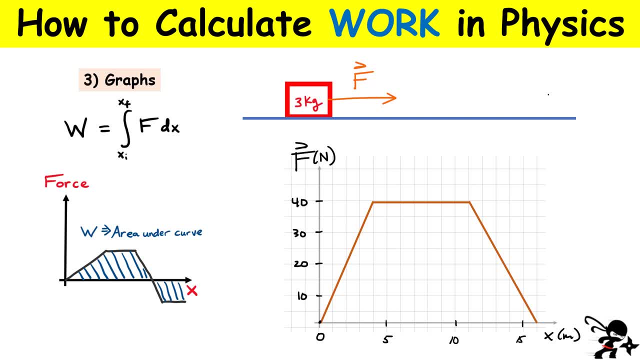 Because the force is always a positive value. In the next example I'll consider what happens if there's a negative value of the force. But right now the force is always in the same direction: At some points it's big, At other points it's a smaller value. 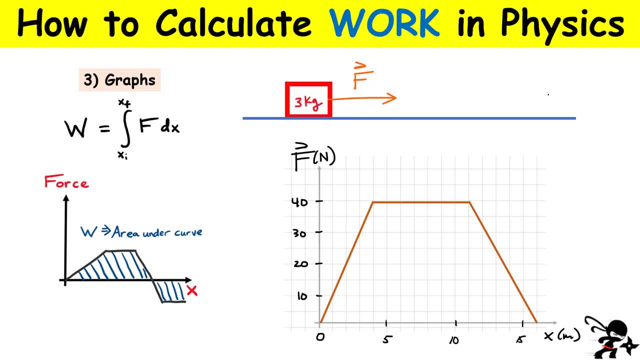 But that doesn't matter. okay, Now, if you're asked to calculate how much work is done by this force, all you need to remember here. now you can write it down as like a calculus problem. But if you don't want to use calculus, you don't have to. 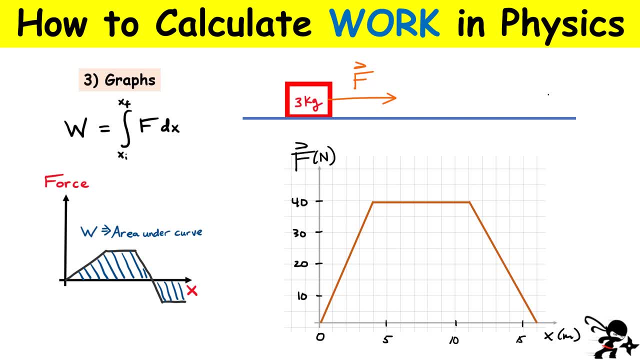 The only thing you need to remember is that the work done by that force is equal to the area under the curve of a force versus position graph. okay, So how would we do it for this problem? Well, again, if you have a more of a complicated shape, 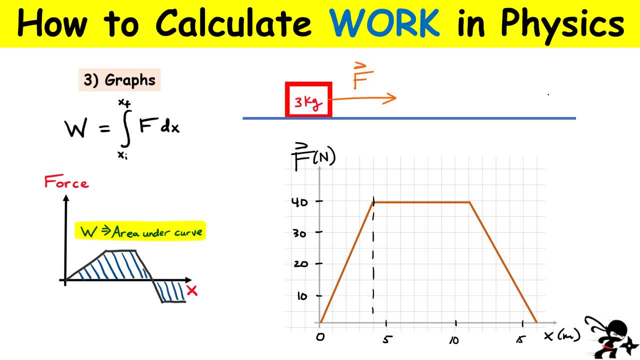 usually what I try to do is I break it down into simpler shapes. I could break this down into a triangle over here, maybe some rectangle over here. right, Call this two. and then another triangle over here. And now for each one of these. 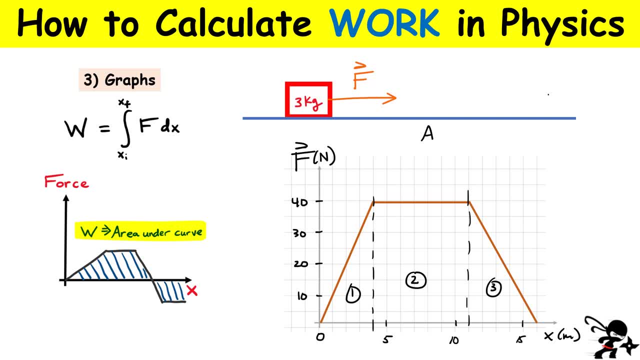 it's pretty easy to calculate the area right. So the area for the first triangle would simply be 1 1⁄2, the base of the triangle multiplied by the height, So you'd have 1: 1⁄2,. the base in this case is four units. 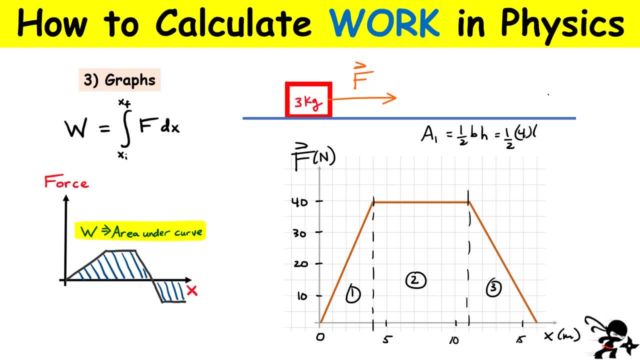 that's four meters and the height is 40, okay, Multiply that through, you should get 80 joules. So in this first part, from zero to four meters, there's been 80 joules of work that was done by this force. 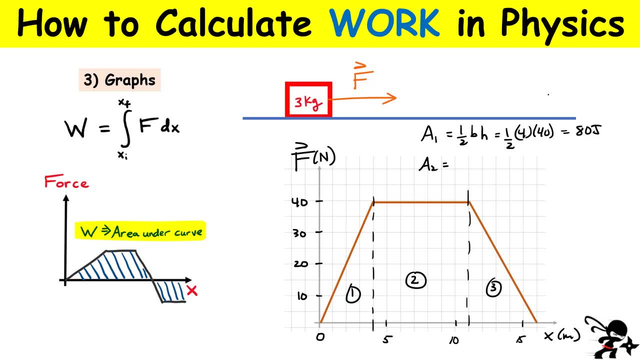 For the second area, that one's an easy one, right, It's simply base times, height, because we have a rectangle. So the base here- just be a little bit careful- that's five, six, seven units, Seven meters is the displacement. 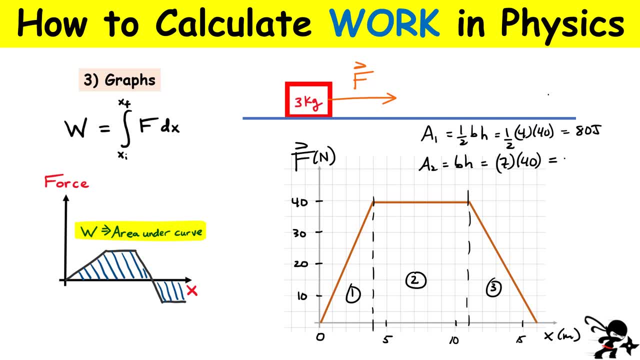 and we have a force of 40 newtons. Multiply that through, you get 280 joules for that section. And then the last one is the third one. The third again, it's a triangle, so 1 1⁄2 base times height. 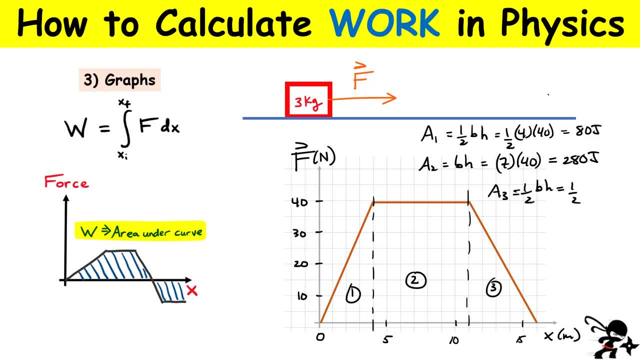 Again, it's 1 1⁄2.. In this case the base is a little bit bigger. okay, It's five meters, And again the height is still 40.. So the area for the third triangle right here should give me it's 200 over two. 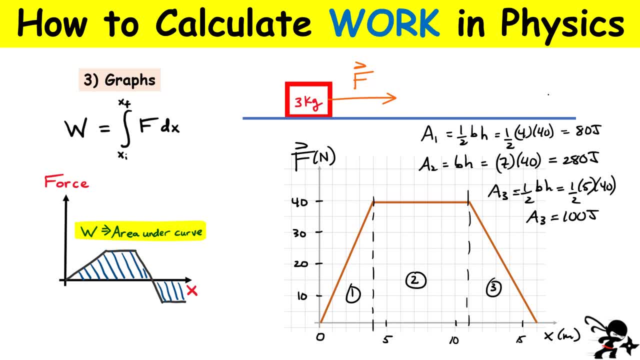 that gives me 100 joules. So if I wanna know the total work, well, guess what The total work is, the total area under the curve- All you have to do is add all of these three up, So 80 plus 280 plus 100, okay. 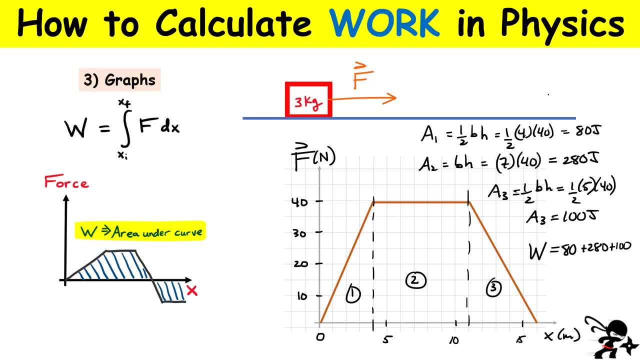 Plus 280 plus 180.. Plus 100, that's 360 plus 100.. The work done by that force F in this problem should give me 460 joules. That's how you would calculate it from a graph. okay, Not too bad. 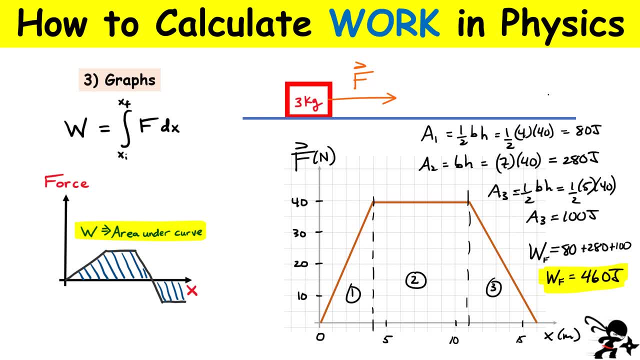 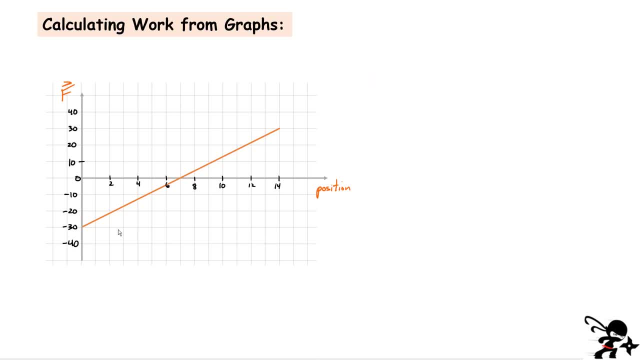 All right, let's look at one last example for a graph and that'll wrap up this video. All right, and the last example here. another example with a graph. just give you a slightly different variation here of force versus position. If I wanted to get the work, for example, 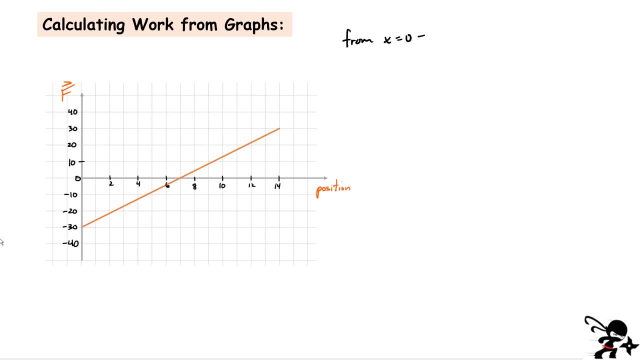 from X equals to zero all the way to seven meters. And what if I wanted to know the work from zero meters, my initial position- all the way to the end, to 14 meters. Okay, so for the first one. again, if you have a graph, 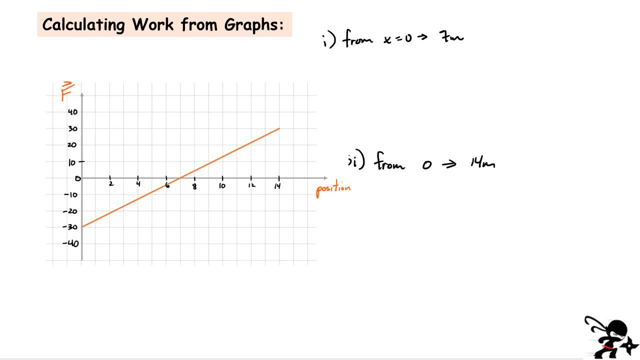 it simply represents the area under the curve. okay, So for this first part, all we're looking for is this area right here. okay, Now what do we do? What do we do with the fact that the force is negative over here? 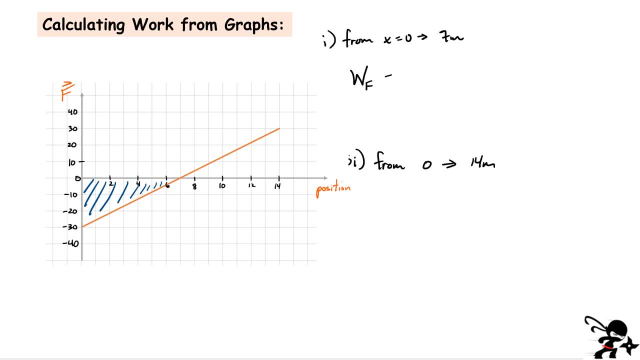 And that doesn't matter. okay, You calculate the work done by that force. Again, it's a triangle. Again, in this case, it's going to be a negative number because my force is in one direction and my displacement is in the positive direction. okay, 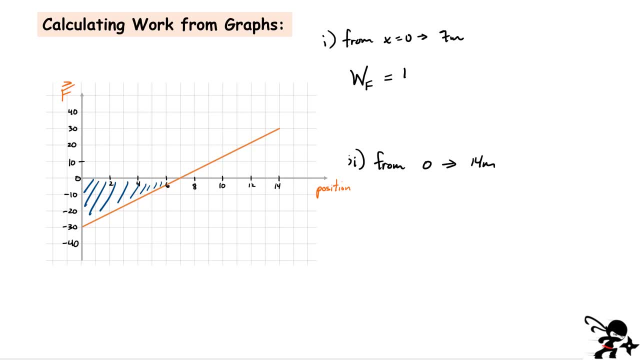 So in this case, here you'd have again just the area of a rectangle, of a triangle, rather. The base is seven meters and the height here is minus 30. Okay, So if you look at that through, you get minus 105 joules. 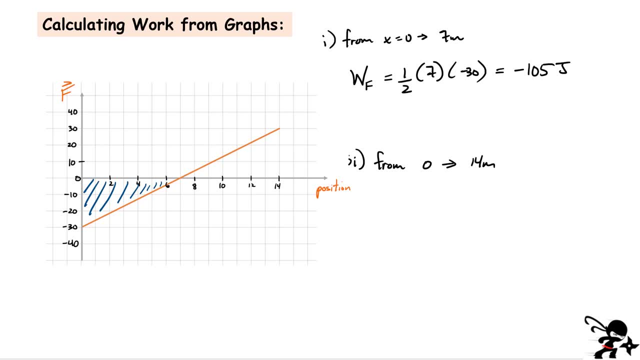 That's how much work was done in that force. okay, How about from zero to 14?? Well then, that's the total area, right? The total area right here is given by this Notice: if this is symmetric here, then I'm also going to have a positive 105 for here. 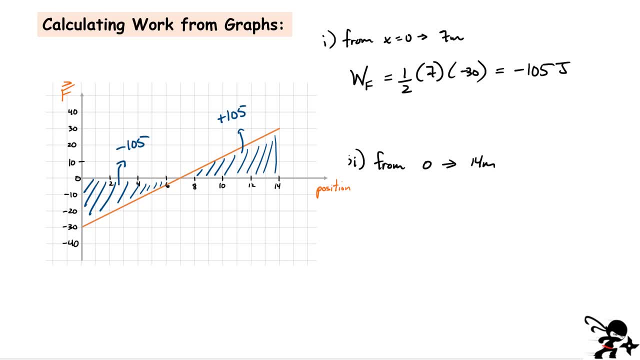 and I had minus 105 for here, right, Because I'm going all the way to 30, and that base is still seven. So that means that the total work done by that force then has to be well, minus 105 plus 105. 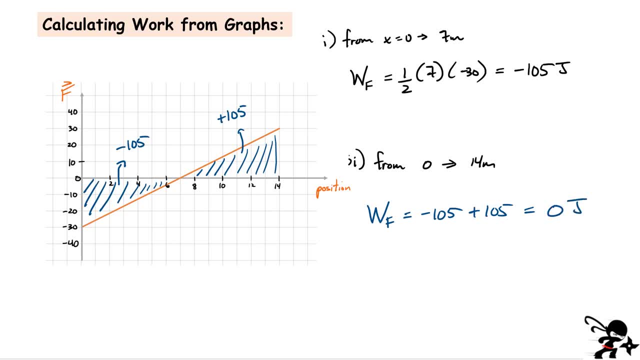 The areas actually cancel out in this case. So there is no net work done by that force over this whole displacement. okay, Over part of the displacement the work was negative. Over the other part it was a positive value and those things can cancel out. 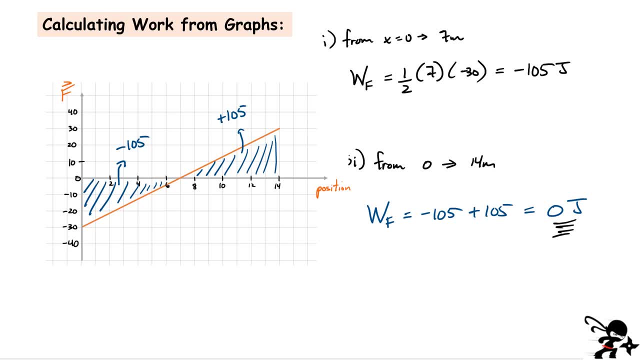 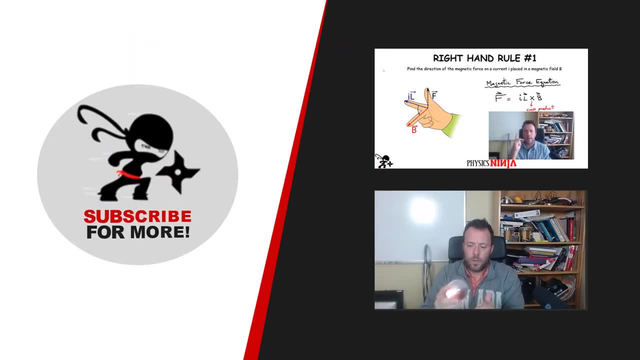 All right, that's it for me, folks, Hopefully you learned how to calculate work for your physics problems. We'll see you next time, Thank you.